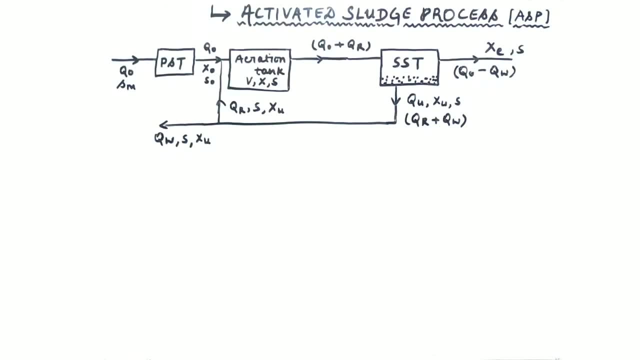 Hello everyone, I welcome you all to my YouTube channel. So this is the most important video of wastewater engineering, which is a portion of environmental engineering. So in this video, we will be discussing the theory related to activated sludge process, which will be helpful. 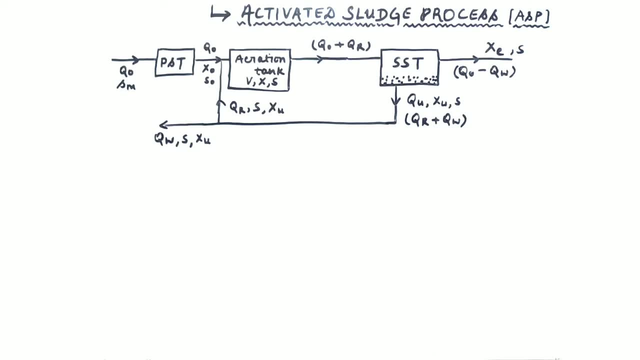 to you in solving the numericals related to activated sludge process. This is very important topic as per the GATE point of view as well as from SSC point of view. In GATE several questions have been framed and in another video I have also solved those numericals. You can also refer 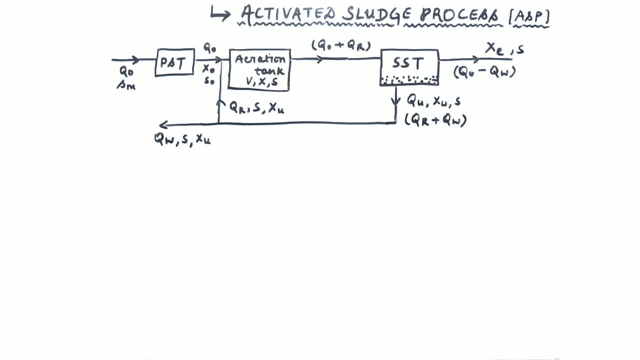 to that video and at the end of the video, you will be confident enough in solving the numericals related to activated sludge process, because I will be discussing in depth this process. So, without any delay, let's get started. See, you all know that in the 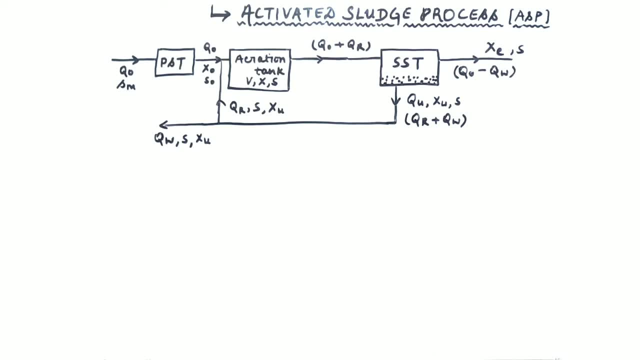 process of treatment of sewage, as well as in the process of treatment of raw water, although we are talking about the treatment of sewage in this particular portion. in wastewater engineering, what happens? There are two processes. One contains the primary treatment and second consists of the secondary treatment. The major chunk of the suspended solids is 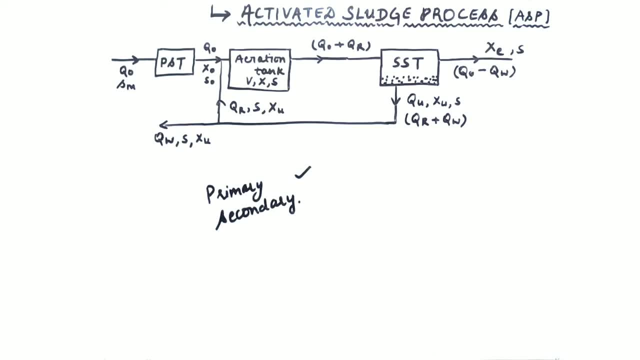 removed in the primary treatment and the major chunk of the BOD or the organic matter is removed in the secondary treatment. This is a very basic point that you all might be already knowing. Second point is that primary treatment also removes BOD. It is not that. 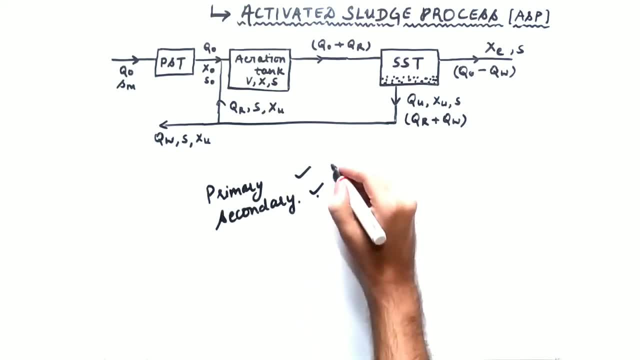 primary treatment will remove 0% BOD. It also removes BOD, but the BOD removed is in minor proportion in the primary treatment, whereas in the secondary treatment solids are also removed. like the primary treatment is mainly for solid removal and secondary treatment is mainly for BOD, 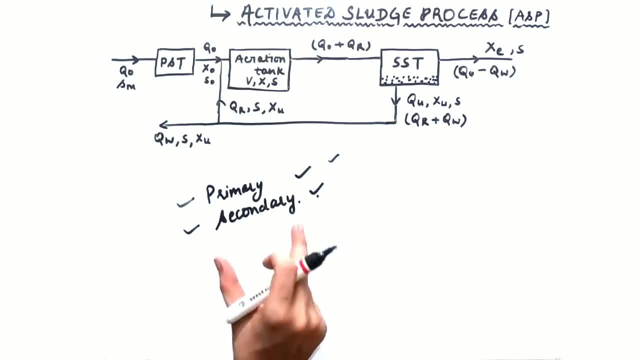 removal, Although secondary treatment is mainly for BOD removal, but still it removes some chunk of suspended solids. Similarly, primary treatment also removes some portion of the BOD, like 40% and something around that. So activated sludge process is a part of secondary treatment and there are 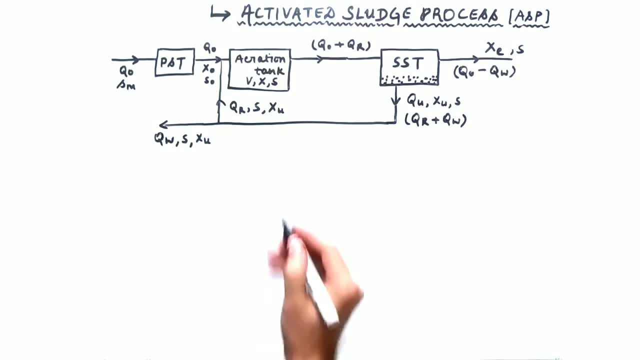 see: secondary treatment means it will be removing the BOD. BOD means the organic content, Organic content means L, So activated sludge process will be removing organic content. How can you remove organic content? Organic content is feeded by the microorganisms. Microorganisms what they do. 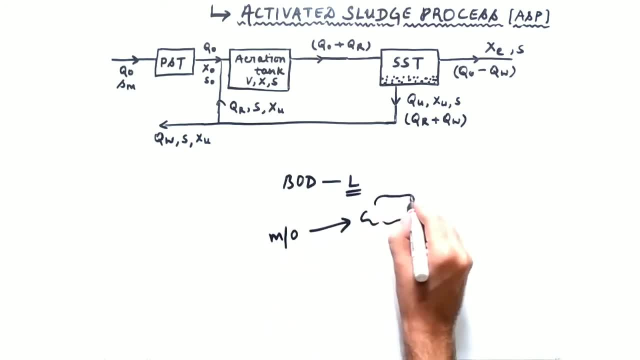 they decompose the organic content, and by decomposing the organic content they reduce the BOD or the oxygen demand for that particular sewage. Now how can you introduce microorganisms? So there are again two methods of introducing the microorganisms. The one is attached growth system, that is called as AGS, and second one is the suspended growth system. 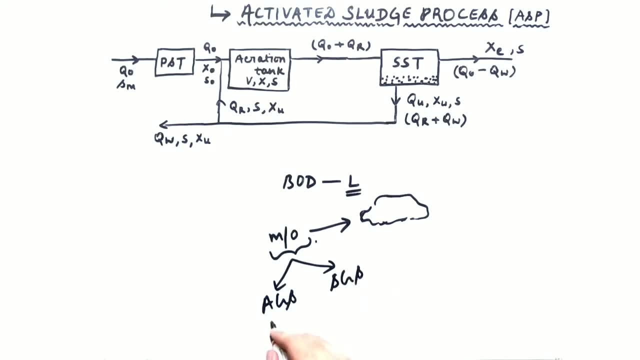 that is SGS. Now you might be wondering: what are what is AGS and what is SGS? So attached growth system is a particular process of secondary treatment used for BOD removal in which the biomass layer, Biomass layer. What does biomass layer consist of? See, by microorganisms I mean. 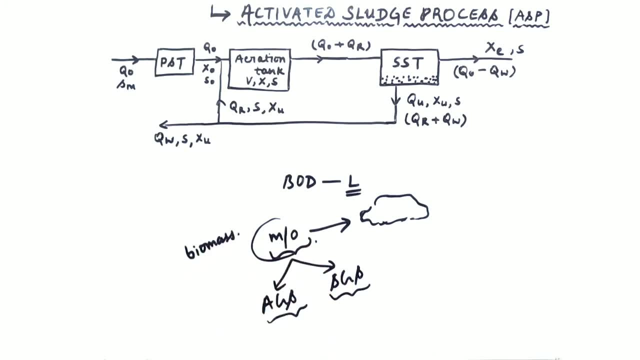 microorganisms. Biomass may not be the actual living microorganisms, but they might consist of, like some decomposed organic matter. Decomposed organic matter: this contains some dead microorganisms. It might also contain some other microorganisms that are dead. Okay, so this is all about. 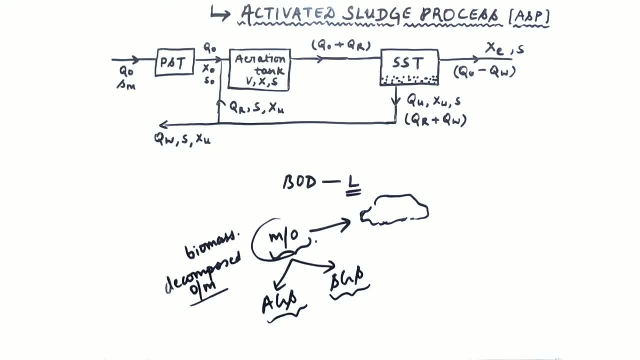 the biomass Biomass is produced during the decomposition and due to the killing of the microorganisms, which depends upon the growth rate of microorganisms. I hope you get this Also. decomposed organic matter contribute to the biomass production. So this is about biomass. Biomass does not directly means microorganisms, but it indirectly means microorganisms. This 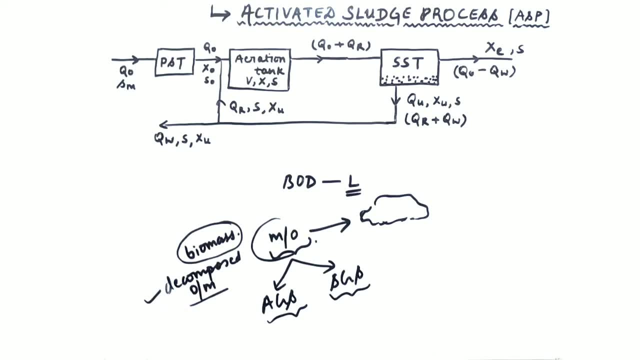 decomposed organic matter will be full of dead microorganisms which will get activated when we introduce sewage there. So AGS is a process in which the biomass layer is grown over a medium over which the sewage is applied. There is one particular medium. Suppose this. 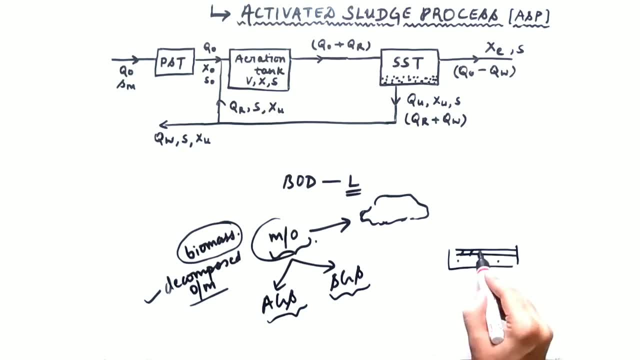 is a medium Here. what do we do? We grow a biomass layer by decomposing the organic matter or by some other means. So if this is a method used to remove the BOD, this is called as activated growth system. Second is suspended growth system. Suspended growth system means: 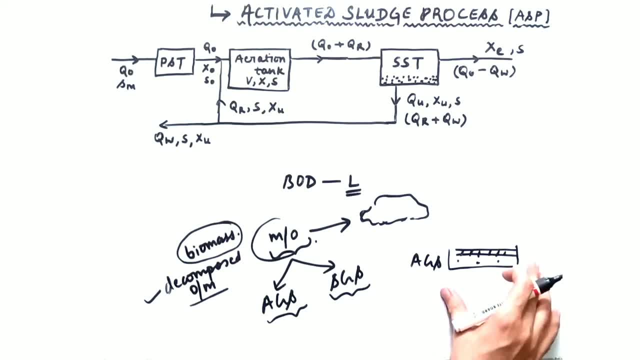 suspended growth system. what do we do? We do not grow the biomass layer. Instead, we apply the biomass over the sewage. The sewage is flowing in some tank and we add biomass here, So this is called as suspended growth system. I hope you get the difference. Activated sludge process is a part of suspended growth system. 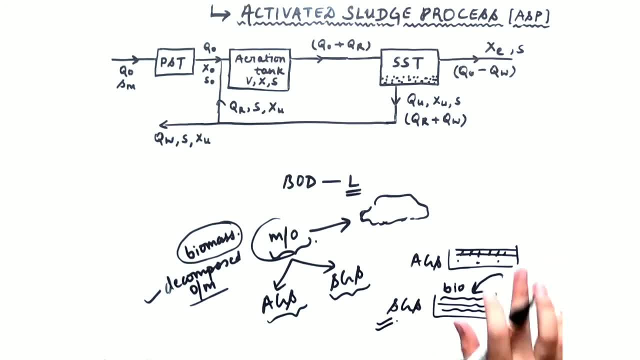 Here we do not directly grow the layer, but instead. what do we do In the aeration tank? The sewage comes from the primary sedimentation tank. after getting the solid settle, The water comes- Sewage water- comes to the aeration tank. 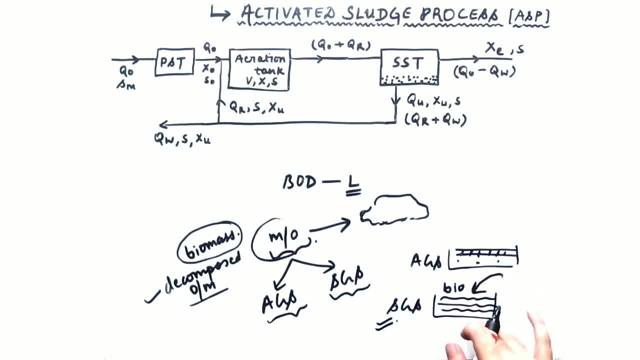 and in the aeration tank we add this biomass layer. from where this biomass layer will come? biomass layer will come from some other tank. suppose this is one another tank. in this tank, what do we do? we fill some organic matter, and this organic matter is treated by some microorganisms or by some other means. 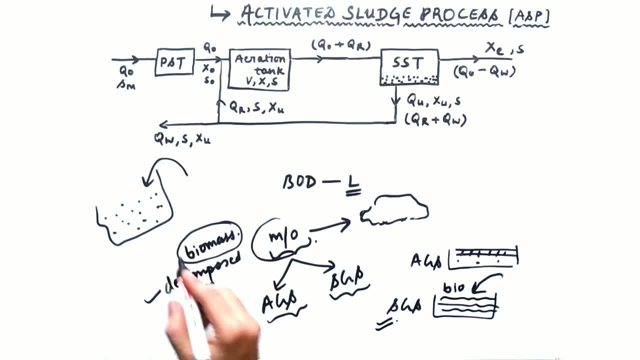 this decomposed organic matter will behave as the biomass. this is what it is called as biomass. biomass is also called as what do we all? biomass is also known as MLSS. MLSS means mixed liquor suspended solids. these suspended solids of organic matter can also behave as the biomass because this MLSS will be rich. 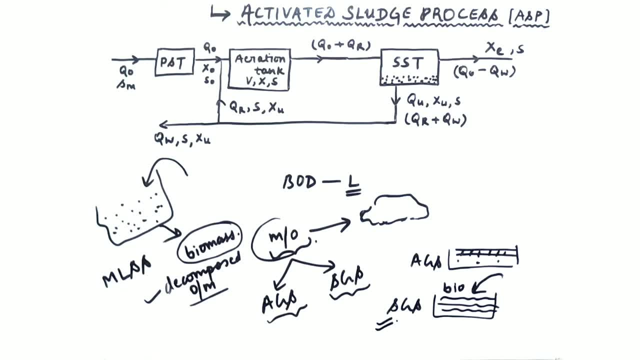 in dead microorganisms which will get activated when the sewage is applied. so this MLSS or this biomass is one or the same thing. this MLSS is applied over the aeration tank. when the sewage comes, the microorganisms get activated. they feed on the organic matter. they reduce the organic matter to some particular value. 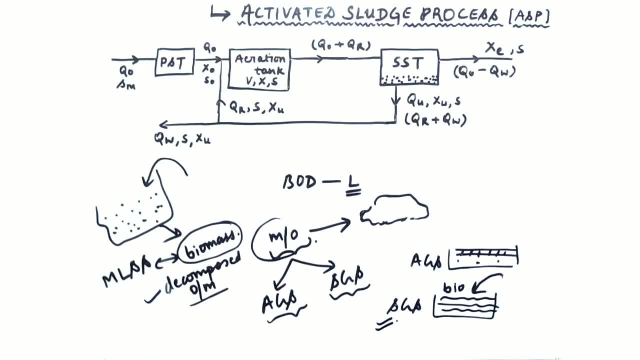 it will not be zero completely. it depends upon volume. so after the aeration tank it goes to the secondary sedimentation tank and from there it comes as a recirculation. so I will explain this process, just wait. so I hope you get what is the meaning of biomass. you get. 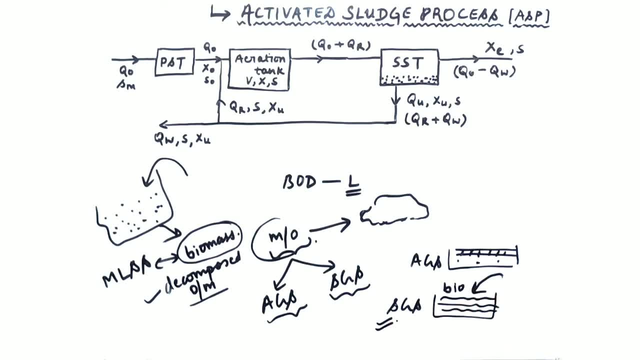 what is the meaning of the concludes the process. just wait, so I hope you get. what is the meaning of biomass. you get what? what is the meaning of AGS and SGS? so now let's come back to the activated sludge process and what this process is. what are these terms? you might be 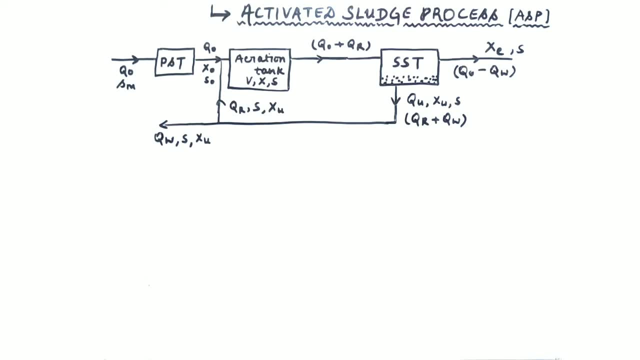 confusing as of now that what is Q naught, what is S, what is XU, what is XE, what is QR and what is QW. but I will be explaining you completely. so just wait, see now what happens. water, first of all sewage water. this Q naught represents. 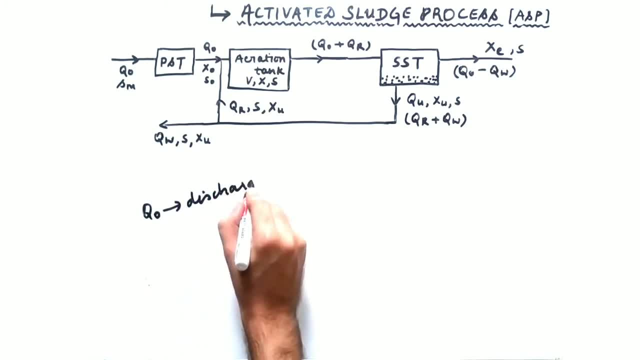 the discharge. discharge can be, in, suppose, liters per day or meter cube per second. this is the discharge, sewage discharge that is coming to the primary sedimentation tank. what is this SM? see, this SM is the food. food means the BOD value or the organic matter or the organic content. this is the organic. 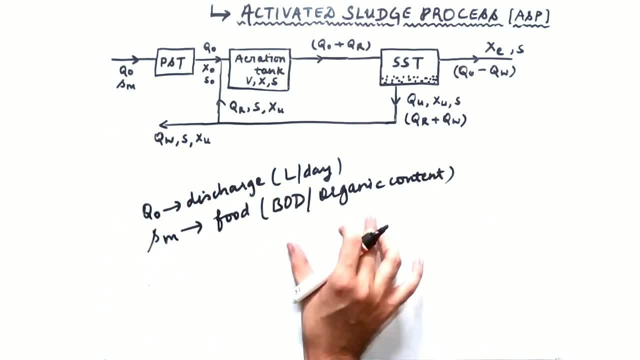 matter or BOD. this is what a microorganism will feed upon. for microorganism, this BOD or the organic matter is food. that is why we depict the BOD or organic content as food in this activated sludge process. I hope you get this. what is SM? 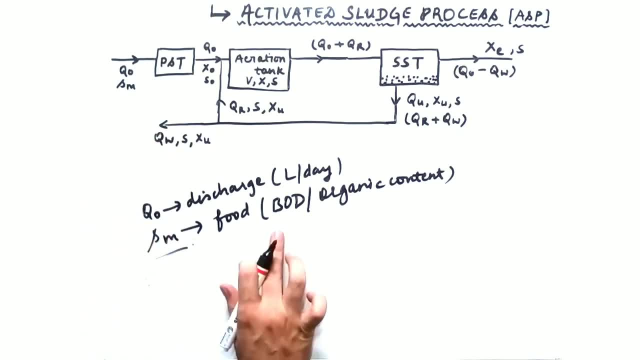 the discharge coming before PST. the amount of BOD present in that is SM. the discharge of that is Q naught. now this Q naught with this SM BOD content will pass through the PST. this SM will have the unit of milligram per liter, just like we talk about BOD. this is 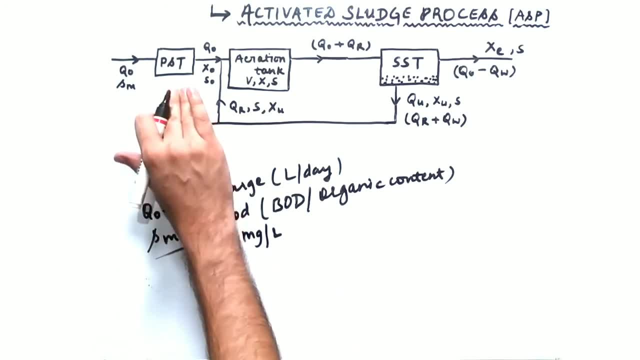 BOD only, but its name is food. this will pass through the primary sedimentation tank. after coming into primary sedimentation tank, its solid content will definitely reduce, although we are not discussing about solid content, because BOD is what matters in the activated sludge process. so its solid content will change, but its food content will also. 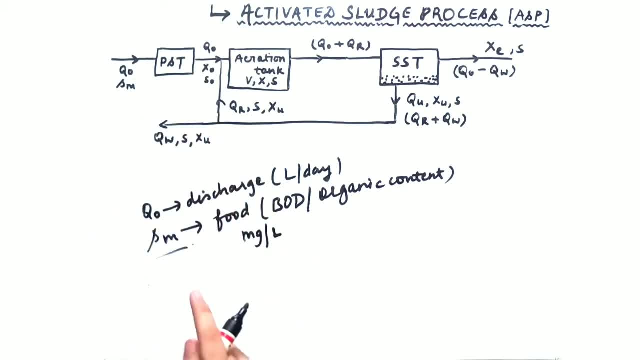 change. that means some part of BOD also removes PST. this is what I started to explain in this video and that is why I said that PST also removes BOD. that is why now BOD will change from SM and will be reduced to S? naught. so the discharge after PST will remain the same, because PST 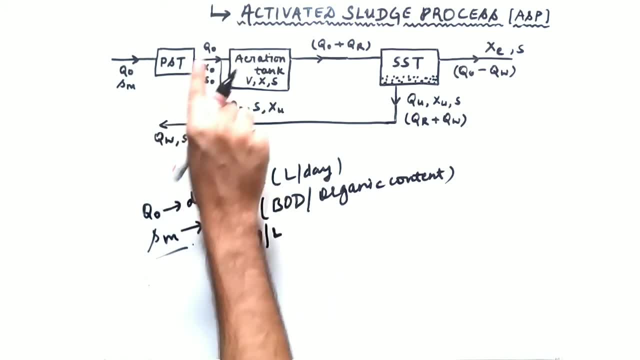 did not eat the discharge. it sent the discharge as it is Q naught, but some part of BOD is reduced to S naught. so now, what is the new food value we have is S naught. now you can also see one more term here, written as excess BOD. 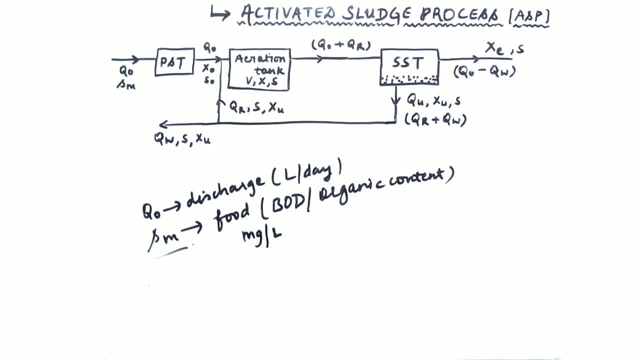 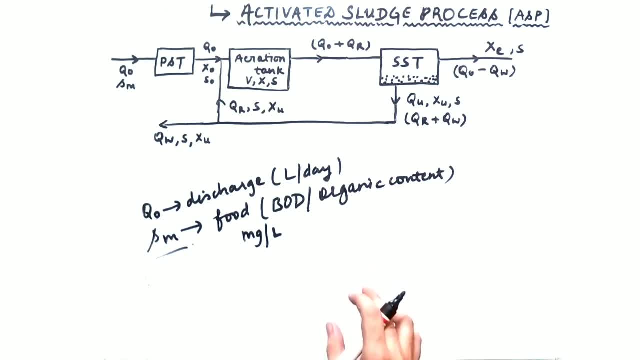 the following ה. we know that excess BOD is a small amount and maximum PST of the food is the quantity of the food being consumed. so this is the amount that we small amount of food. with extending campaign it is remaining low. What is excess BOD? The amount of digested and excretory products is less than FOD- some have to be taken care of- and the amount that the stock is taking tuck because the composting products will not be heavenly delicious- which is already present in the sewage. 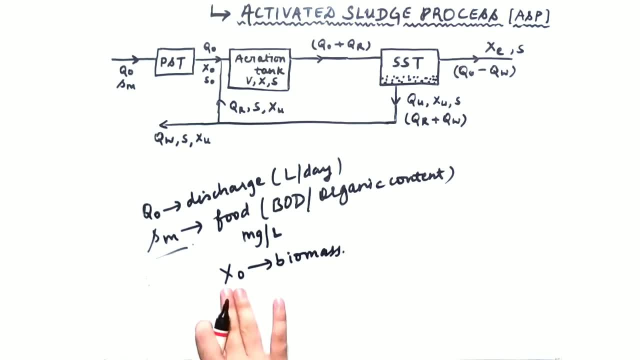 However, when you read the assumptions, then you will come to know that the biomass of the incoming sewage is neglected. That means we consider it as 0 mg per litre, But this is just an assumption. In the question sometimes the examiner 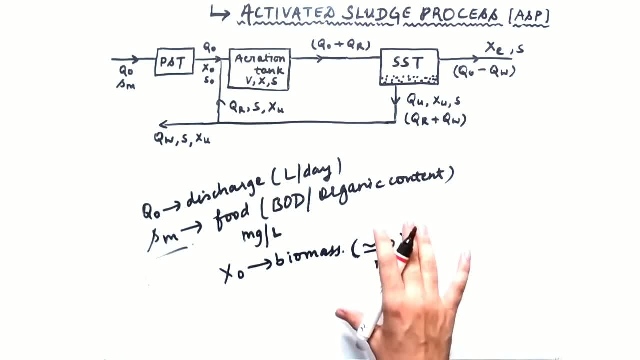 may give you some particular value for this biomass that the content of the microorganism is already present in it. I hope you get what is the meaning of Q0, S0 and X0.. Now, what matters to you are these three values. 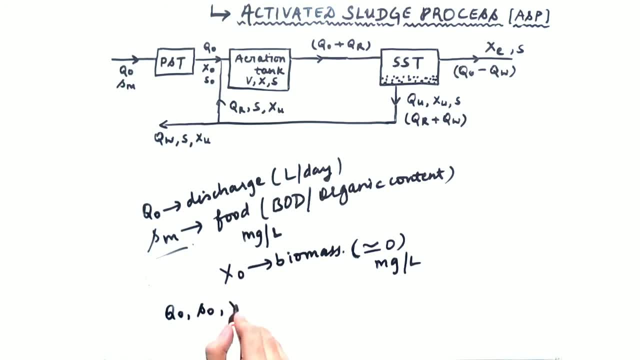 Q0 is present in the aeration tank, S0 is present and X0 is present. Q0 is the discharge, S0 is the BOD which is present in the aeration tank. This is called as effluent sewage, The sewage that matters for you. 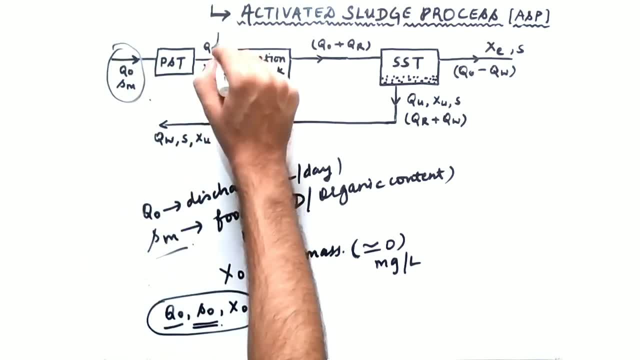 does not matter for this one. This is going to PST. This sewage matters for you. What is this sewage? It will be called as influent sewage. This goes to the aeration tank. Now the entire process of BOD removal happens only in the 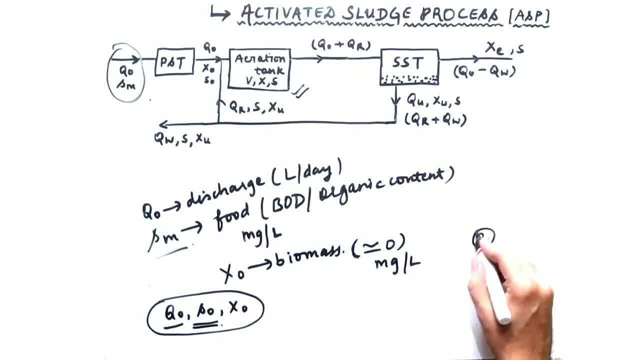 aeration tank. This is your second assumption, that the entire process of BOD removal happens completely in the aeration tank. Now, what is V, What is X, What is S? This is what I have made in the aeration tank. 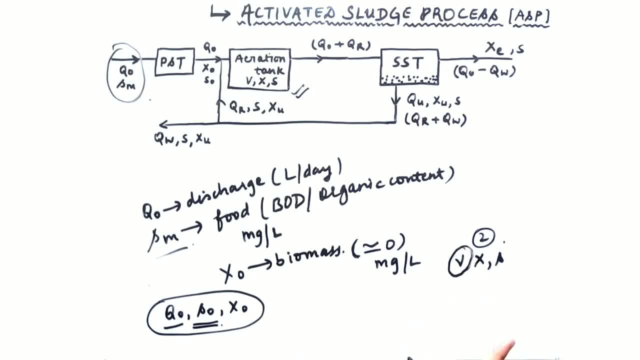 V is the volume of the aeration tank which you will use in the formulas. The higher the volume of the aeration tank, the better it is for you, because the better your BOD removal will be. So V is the volume of the aeration tank. 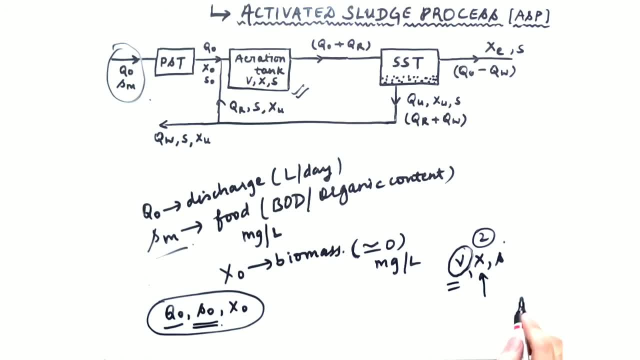 What is X? I had told you that this is a suspended growth system. So when sewage comes here, you add a biomass layer to this aeration tank. So how much biomass are you adding to this aeration tank? That is our X. So basically, 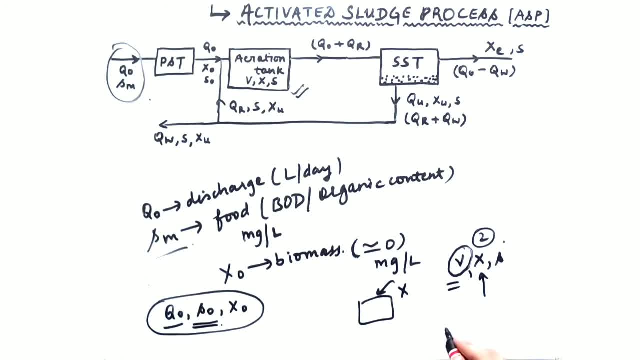 we can call X as the biomass content in the aeration tank, Although this is not present in the aeration tank. We are not growing a layer. If we would have grown a layer, it would have become an activated growth system. We are suspending a layer of. 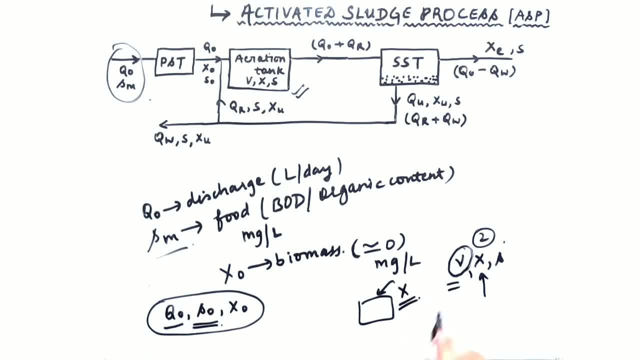 biomass with the content of X. This X is the biomass content that we add in the aeration tank, or we can say that it is present in the aeration tank for the time being. What is S now? S is never present in the aeration tank. 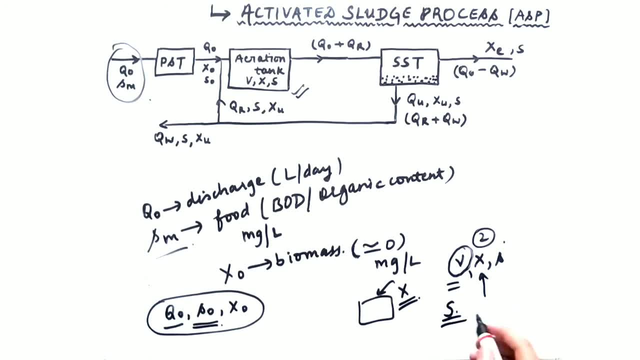 When the process of S in the aeration tank is over, the amount of BOD that is left is called S. Let me explain you. This is your aeration tank. From here you are getting the discharge of Q0, S0 and X0. 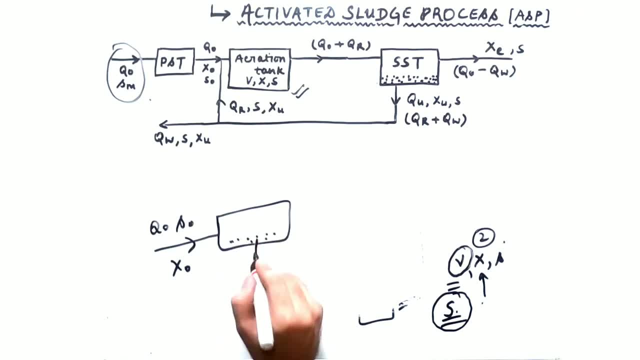 Now, since we have added microorganisms in the aeration tank, and these microorganisms are called biomass and MLSS. Its concentration is X, its volume is V. When this biomass layer will decompose on this sewage and reduce its organic matter, then the final BOD that is left. 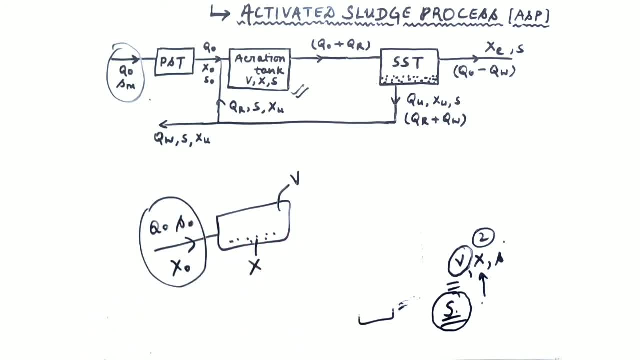 in the sewage will be S. All the microorganisms have fed on all the sewage according to their capacity. After that, the final BOD of the sewage water is called S. So I hope you get it now. S is the BOD. 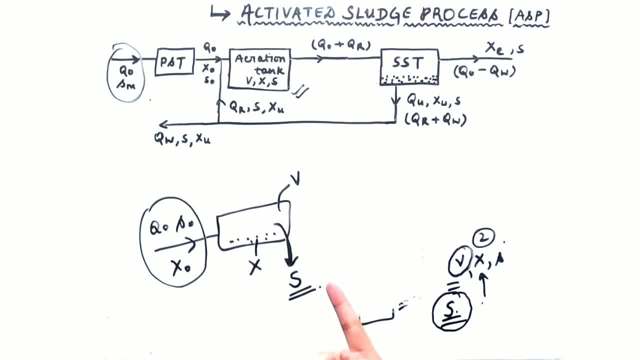 or the food or the organic matter of the treated sewage in the aeration tank. Now what happens? Some of the sewage will come back. Q0 will definitely come back, but we will do one more recirculation. Now why is recirculation done? 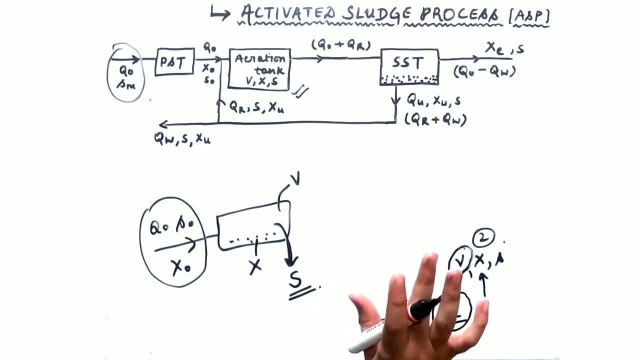 First I will tell you about recirculation later. Now assume that some recirculation has been done from here, due to which Q0 has become Q0 plus QR. Now Q0 is coming from the aeration tank, which was the original discharge. 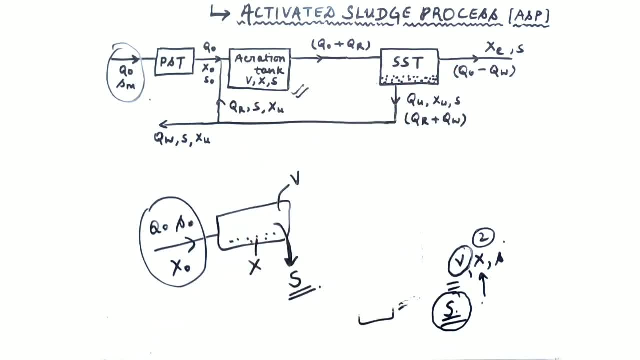 of the sewage water, The water which will come out from here, the BOD of S. along with that, some of the biomass layer also comes along with it. When the sewage water travels, some dead microorganisms or biomass will also travel along with it. 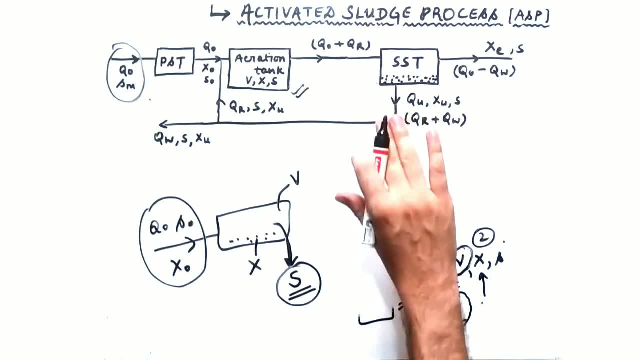 They will settle in the secondary sedimentation tank. Along with that, some solids will also settle in the secondary sedimentation tank, So that biomass plus the solids will settle in the secondary sedimentation tank, and this settled sewage is called as sludge. 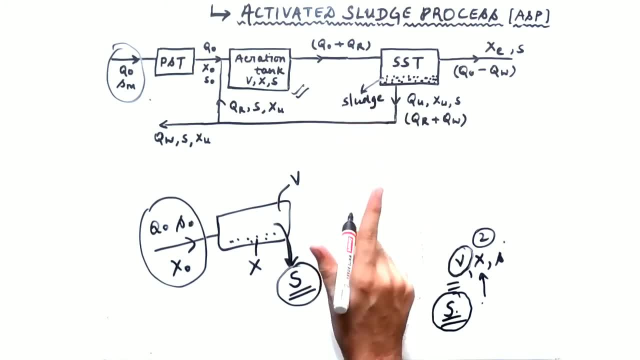 This is called sludge. This is rich in biomass concentration because from here all the biomass will settle down. There are solids in it, but as much as biomass will go up from here, all of it will settle down. This is why this sludge. 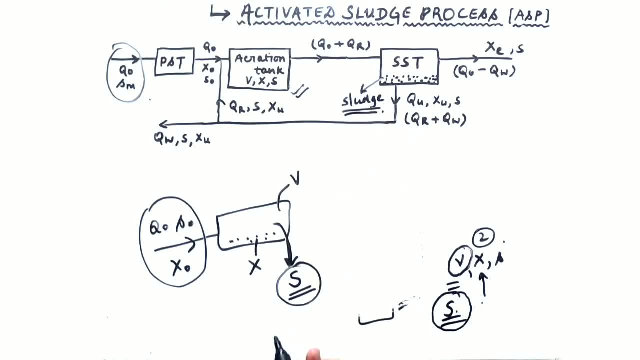 is rich in biomass or the MLSS concentration is very high. Now, from here, your Q0 minus Qw discharge will go from the secondary sedimentation tank. Initially your Q0 discharge was going, but your final is going to Q0 minus. 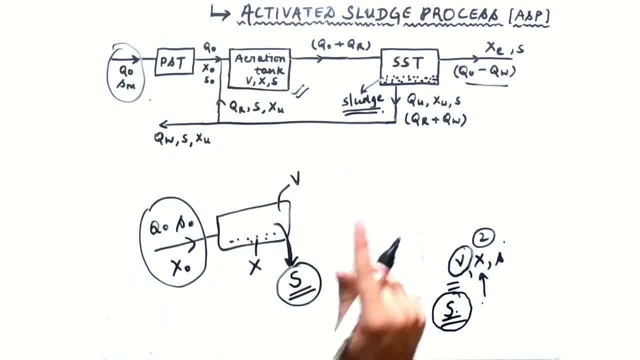 Qw because we waste some discharge. So from here, Q0 minus Qw discharge will go. This discharge is the floating water part of the sewage. Now this discharge that has passed from the secondary sedimentation tank is now our clean sewage, Although 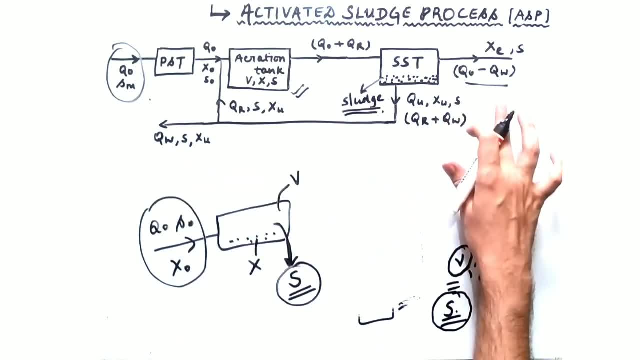 some of our discharge has been lost, but still we got a major chunk, which is our treated sewage. So Q0 minus Qw will come out of the secondary sedimentation tank. Now see, the food will remain same in the sewage as it was in the BOD. 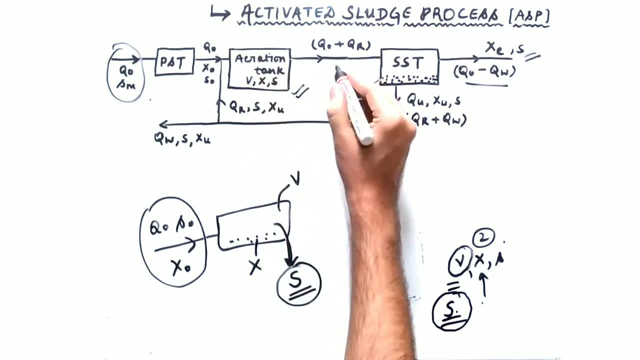 So the sewage that came from here is also our BOD and the food is the same, And the food that came from the secondary sedimentation tank is also our BOD and the food that will go out will also remain the same, But this is our Xe. 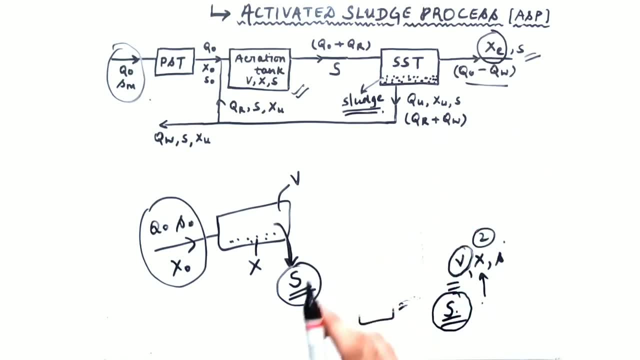 What is Xe? I told you that we had biomass concentration. So because all the biomass was settled, the floating sewage has a very light MLSS, which means very light biomass is left here. So the concentration of biomass in the floating sewage. 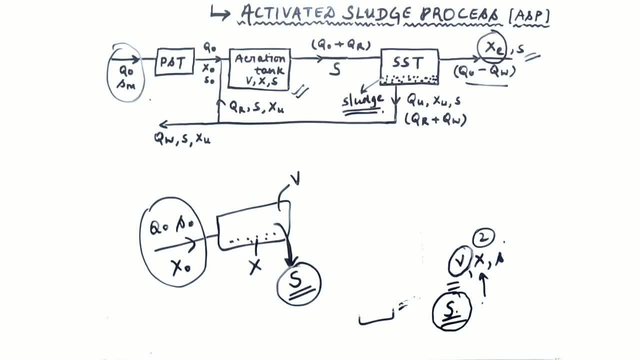 is Xe. So whatever discharge is coming out from the secondary sedimentation tank, first of all it is Q0 minus Qw. It is a little wasted and reduced. Second thing: the food from here to every point will remain the same after the food. 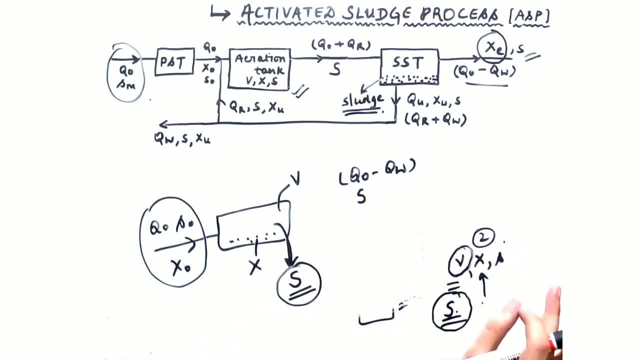 is in the BOD. The concentration of BOD will always remain the same. The second thing is our MLSS concentration, because all the MLSS has settled in the form of sludge, So the floating MLSS concentration will be Xe, Although we assume. 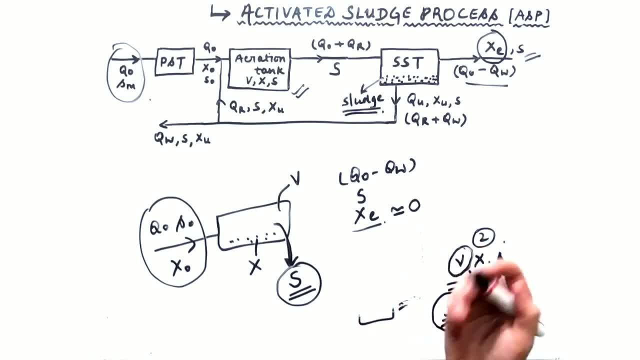 that it is also almost zero. But in the question, even if it is not zero, it can give some value of 20mg per litre or 30mg per litre But its value will be very less, But the value of the Xe in the sludge. 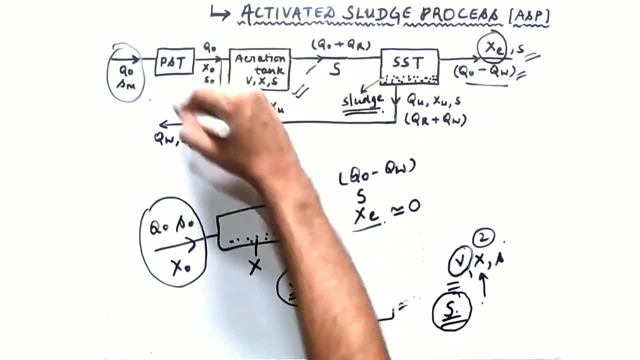 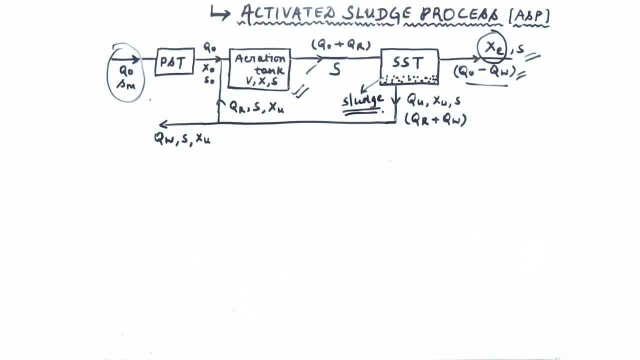 will be more. I hope this point is clear. Now we will talk about the recirculated discharge from the secondary sedimentation tank. Now see what happens In the aeration tank. we have to maintain the food by biomass ratio, which we call F by M ratio. 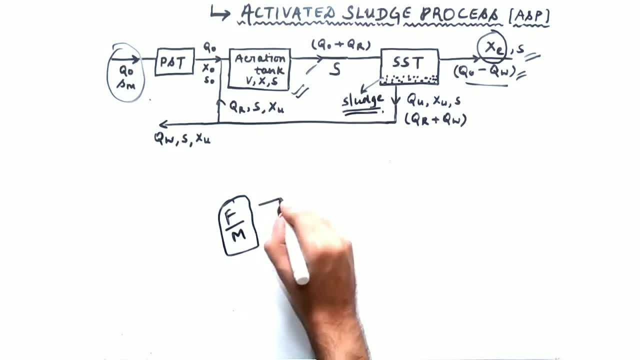 We have to maintain the food by biomass ratio. What is food? Food is BOD. What is biomass? Biomass is the micro-organism. This is our main funda that we have to maintain the F by M ratio in the aeration tank. 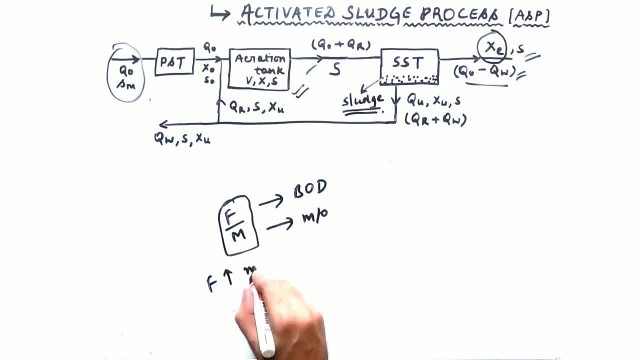 If we have more food and less micro-organisms, then our process will be bad. We have more BOD, but to decompose it we have less micro-organisms, So our process will be bad. So our F by M ratio should not be less. 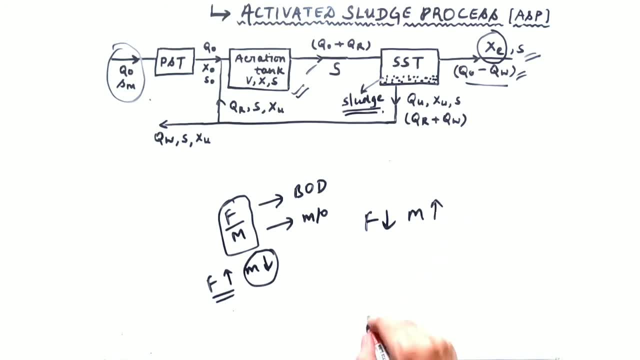 Now, if we have less food and more micro-organisms, then the micro-organisms will be more. There will be scarcity of food. Micro-organisms will react with each other and will feed on each other. This will destroy the layer of micro-organisms. 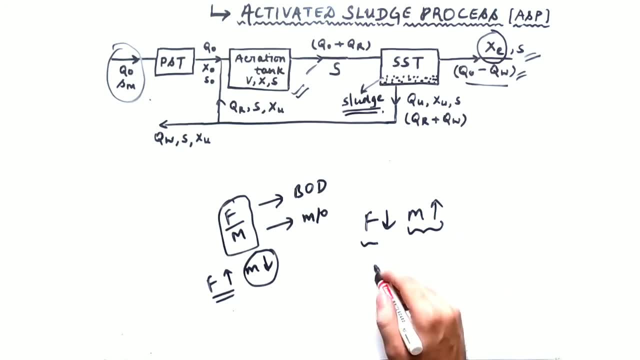 The food that will come will not be decomposed Here. also our process will be bad. So our F by M ratio should be optimum Because of this. what do we do To optimize the F by M ratio? we do two things. 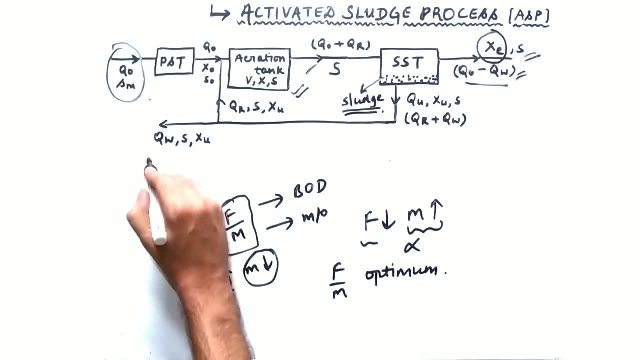 One we do recirculation And the other we do QW. We waste any discharge. Now see if the ratio increases. that means the biomass concentration in the tank is less. We have less biomass concentration. Our F by M ratio has increased. 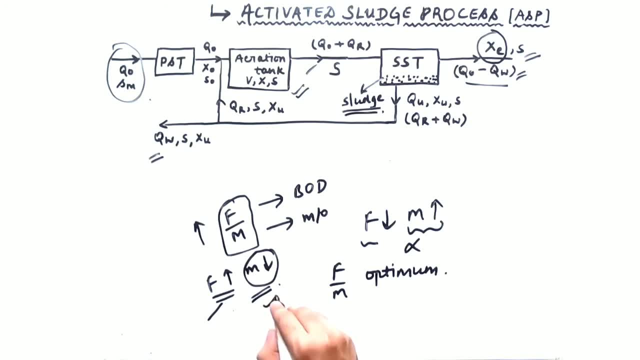 If it increases, then the food will be more and the biomass in the aeration tank will decrease if our F by M ratio increases. In this case, what will we do? We will recirculate the discharge By recirculating the discharge. 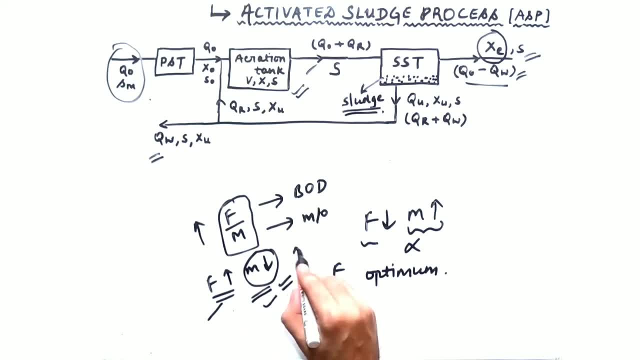 the content of the micro-organisms will increase again. This will make our F by M ratio optimum. I told you, the sludge that settles in the secondary sedimentation tank is very rich in biomass. All the biomass that comes from here is settled. 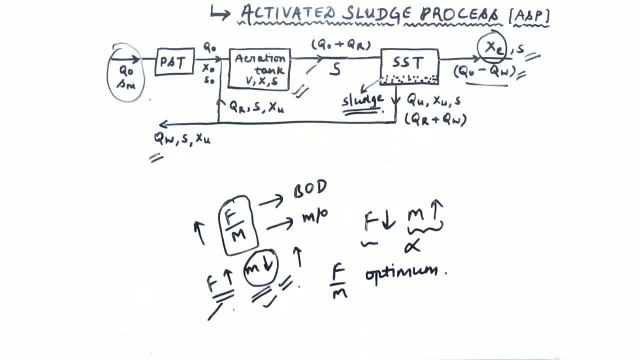 So if you recirculate the sludge in the aeration tank, then what will happen? The recirculation takes place in the aeration tank. So this recirculation will happen because of the recirculation of sludge. 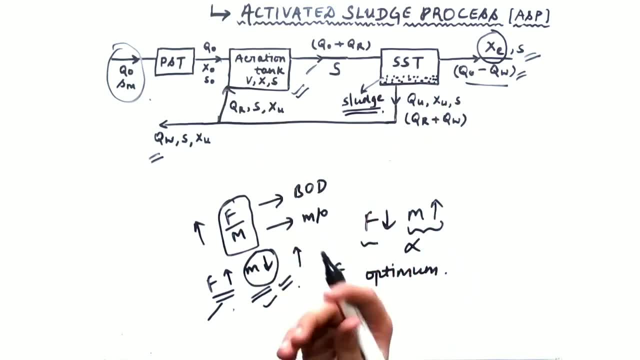 To recirculate the sludge, you have to recirculate the biomass. in the secondary sedimentation tank The micro-organisms increase because of the recirculation. We have not changed the food, but the biomass will be affected. So the F by M ratio will be optimum again. 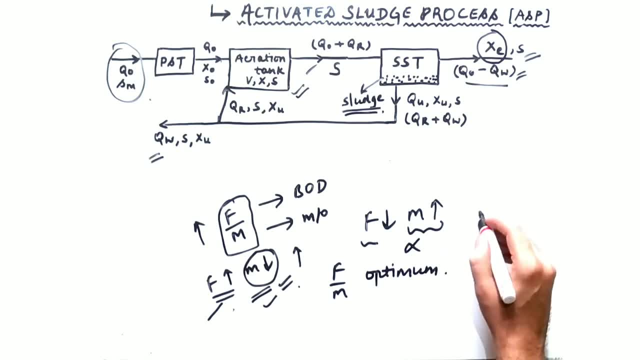 So we have recirculated the sludge. The second case is that the F by M ratio decreases. If the F by M ratio decreases, it means that the micro-organisms increase and the food decreases. So we have to reduce the micro-organisms. 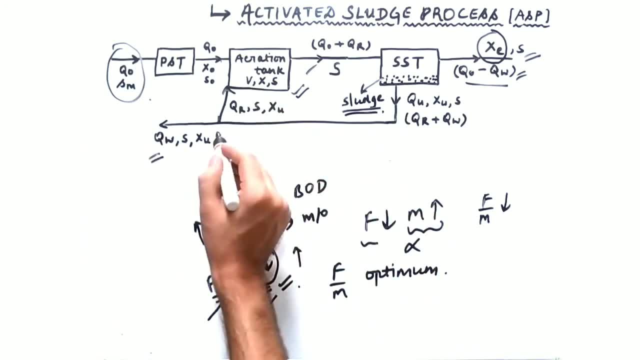 So we will waste some discharge here. What will happen? The content that was going will decrease, The micro-organisms will decrease, The M will decrease, The F by M ratio will be optimum again. So we have wasted here. So these were the two processes. 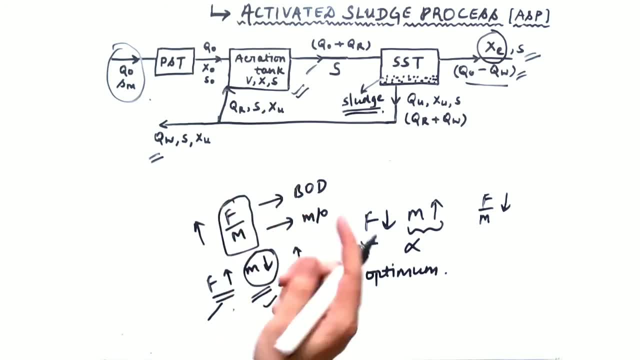 of recirculation and wastage. Why is recirculation done To optimize the F by M ratio? Why is wastage done To optimize the F by M ratio? When the F by M ratio increases, we do recirculation. 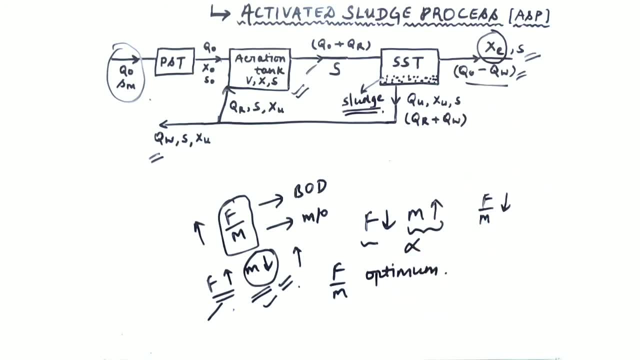 Because the F by M ratio is much more So. the F by M ratio is much more So. this is what we have seen. That's where the final discharge that came out was Q0-QW. Now see, Q0-QR is coming from here. 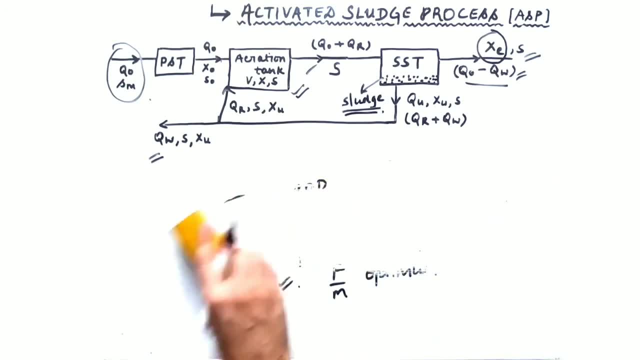 and Q0-QW is going from here. So how much will go here? Q0-QR is coming and Q0-QW is going here, So you can apply mass conservation simply How we have to get the value of r from plus. 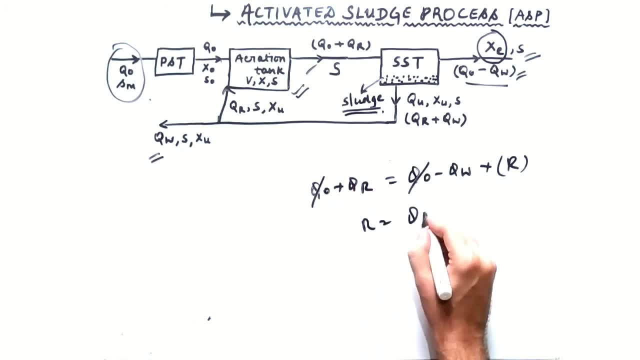 so what will be r? q0 will be cut from q0, so qr plus qw. this discharge will recirculate from here. this is the value of r, this is coming and this is going, and this is also going, so you can simply apply the rule of conservation. 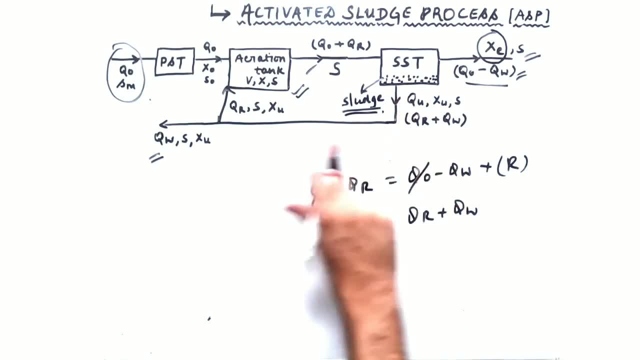 so you will get this value. so the discharge that will go from here is qr plus qw. we can call it qu. we called addition as qu. what is xu and s food will be constant everywhere. when it came it was s0. after leaving the aeration tank. 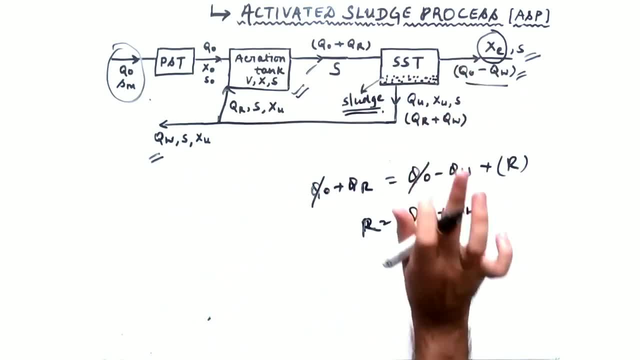 the value of food will be s everywhere here. the concentration of biomass is xu here. I told that it is xe. why is it xe? because floating is very less so. it is xe here it is xu. what is xu? because sludge is being circulated from here. 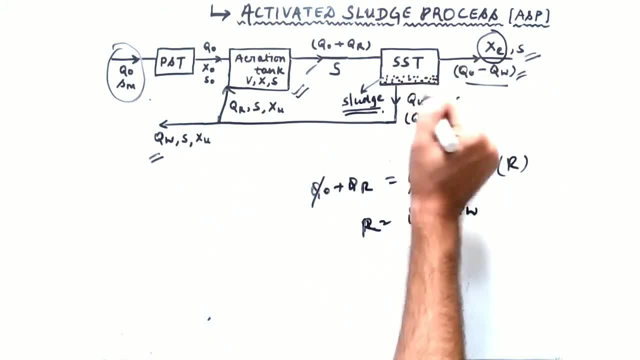 the water of sewage is being circulated here. the sludge is lying down here. we have circulated it here, so now this sludge is very rich in biomass concentration. because of this we have taken it separately. here biomass concentration is xu. here biomass concentration is xe. here biomass concentration is x. 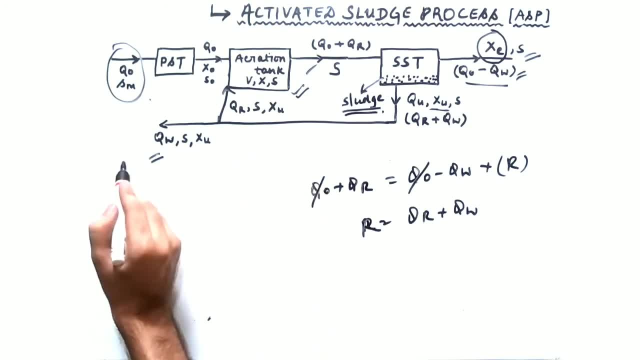 ok, this is recirculated. here also we are wasting the same recirculation discharge and here we are recirculating. so here will be xu, here will be xu, here will be s, here will be s. so this diagram should be made in your mind. you should know that. 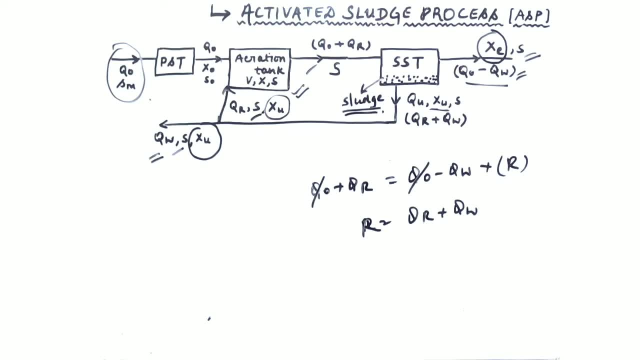 where s is, where xe is, where xu is, where x is where q0-qw will go. where qu will go here, qr will go here, qw will go. when qr goes here, q0 plus qr will give you q0 plus qr. I hope this diagram is clear to you. 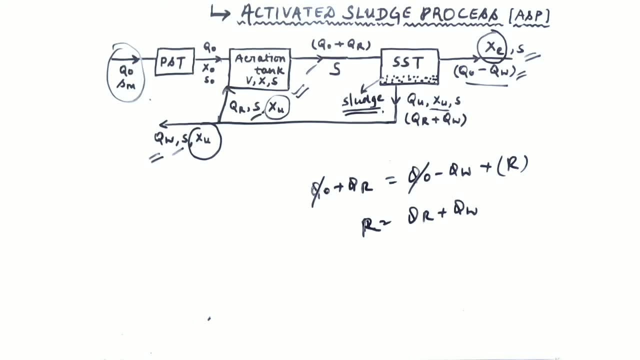 now you have some formulas. if you have clear diagrams, then these formulas are very simple. now let's look at the formulas. so very first formula is Detention Time, time which is called as TD, or it is also called as hydraulic retention time. remember this, so you know that Q equals V in the aeration tank. 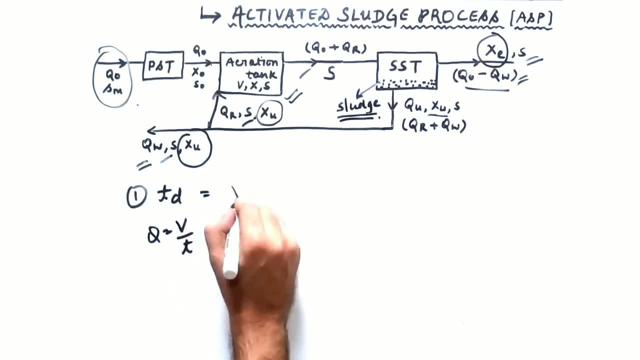 that's why TD equals to V volume of the aeration tank divided by aeration tank divided by Q0. so that's why TD is V divided by Q0. as simple as that. second point. second point is sorry, organic loading rate. what does organic loading rate mean? 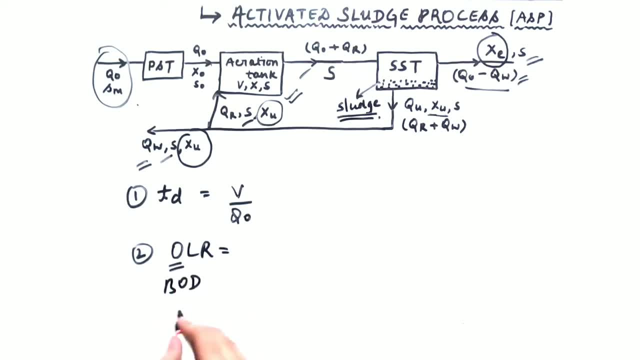 organic means BOD, organic content being BOD, Wheatting BOD S. So how much S you are applying in the aeration tank? so how much organic loading rate? and if you remember from another video in which we can see about trickling filter, in it we saw organic loading rate formula, that is胡 0, Sud 0. 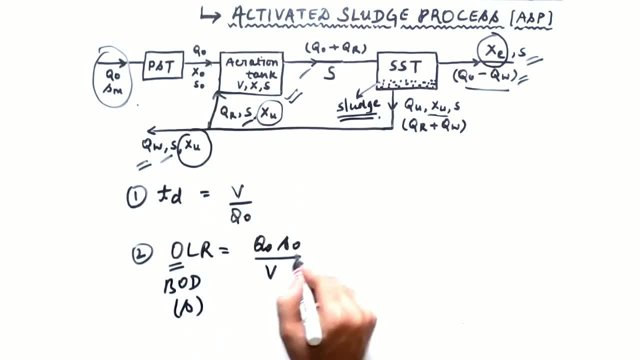 that is q0, s0 divided by b0 divided by V. What is Q0? How much discharge is coming and what is S0? How much BOD we have applied means how much is the BOD content of the sewage. So Q0 into S0 will give you. 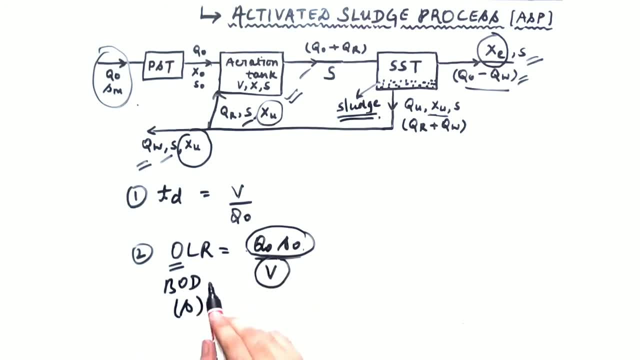 the food content divided by volume. Organic loading rate is per unit volume. hydraulic loading rate is per unit surface area. So what will be its units? So units should be remembered: kg per day per m3.. So this is the organic loading rate. Now you don't have. 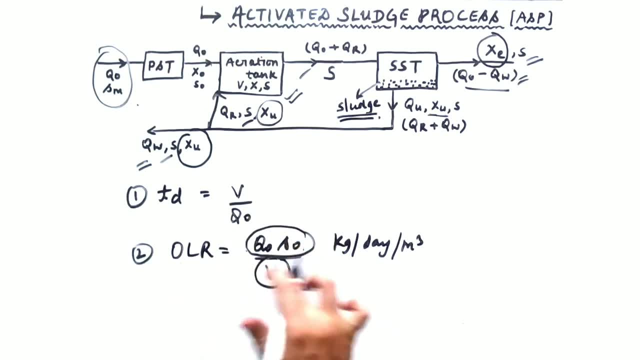 to remember all the formulas. Now you know about every term. All this is going on in the aeration tank. What is coming in the aeration tank? this is what we are loading. How much sewage are we loading in the aeration tank? Q0 into S0 means basically how much. 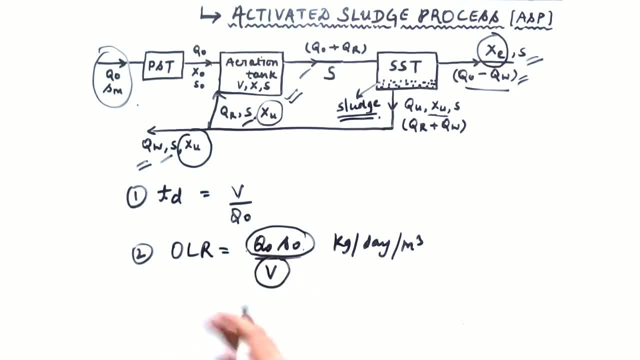 organic content. are we loading, That is, Q0 into S0 divided by volume? Third point: specific utilization rate. Specific utilization rate. What does this mean? Specific utilization rate means this is the ratio mass of the BOD removed to the mass of the. 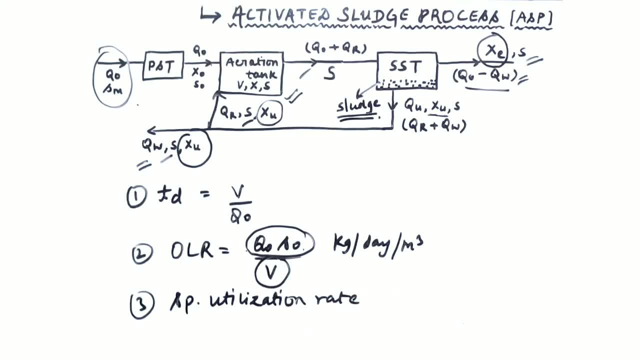 BOD removed. This is the ratio mass in the aeration tank. We had applied some biomass. This is our biomass. What did this biomass do? It fed some BOD. So let's see this utilization. How much of this biomass has utilized BOD? It is a CBC thing. So where is the work of 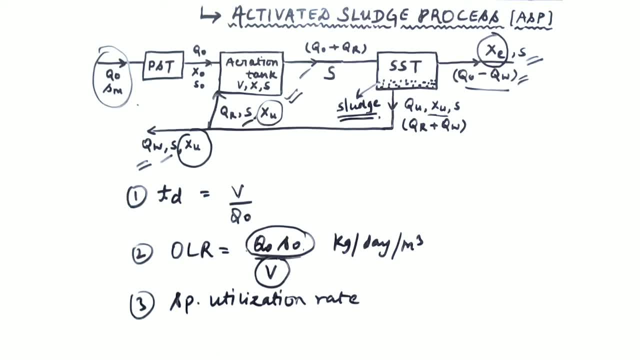 biomass going on? It is going on in the aeration tank. And where is the food utilization going on? It is also going on in the aeration tank. So what will be the formula for this? Q0? S minus S0, divided by BFC? How did this come? Q0 is the discharge, S minus S0.. S is your. 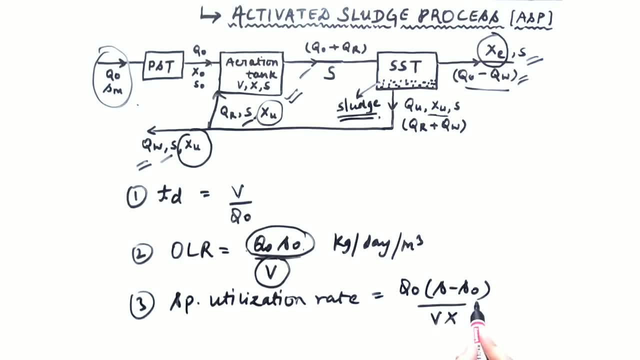 food initially BOD and S0. sorry, S0 minus S. This will be S0 minus S divided by BS. What is S0?? The food that is initially coming to you that is initially BOD S is the final that is coming out of this. After the complete treatment, this much BOD is left. So how much? 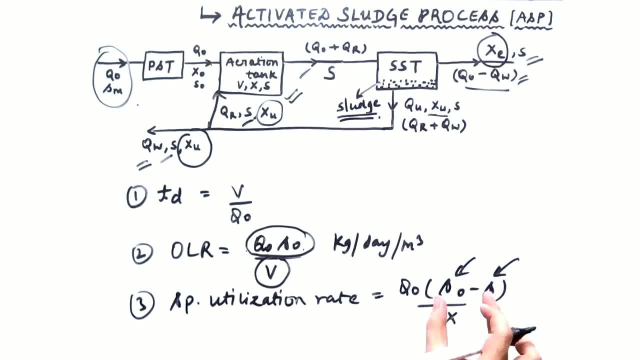 BOD was utilized. S0 came and S went, So how much use did the biomass do? This much BOD was consumed. So S0 minus S is the BOD used. How much was the discharge? This is the BOD. 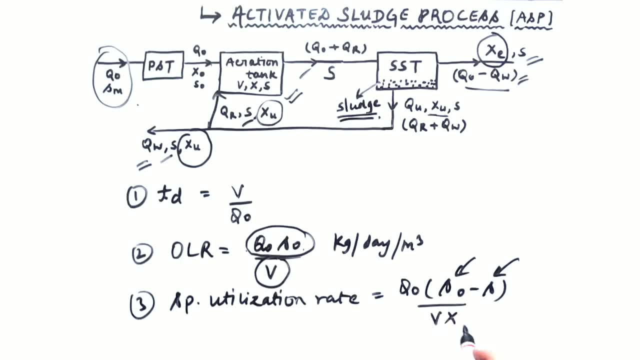 How much was the discharge Q0 multiplied by this? How much biomass was used? This is V into X. What was X Concentration of biomass that was feeding on this? What is V Volume? So if we multiply it by volume, then this unit will be less. There will be no unit. 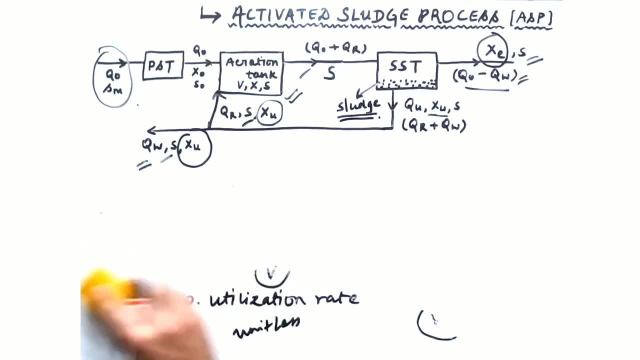 of this. These three formulas are clear. Let's move on to the next formula. What is the next formula? We have recirculation ratio, Recirculation ratio. So this is very simple: Recirculation ratio. So you are reading in the environment: QR divided by Q0.. Now there is a derivation. 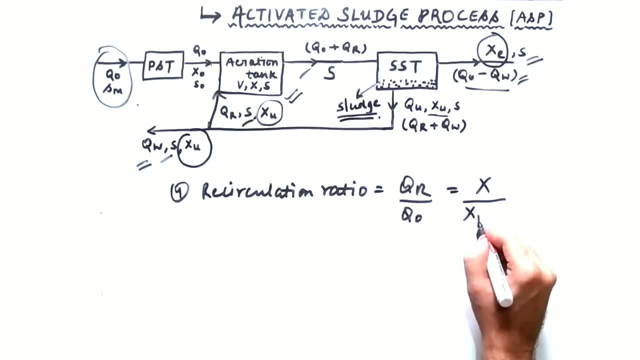 of this, in which I will not go because it is a little detailed, So you can remember it directly: QR upon Q0 is equal to X divided by XU minus X. What is X? The concentration of biomass in the aeration tank? XU is the concentration of biomass in your recirculated. 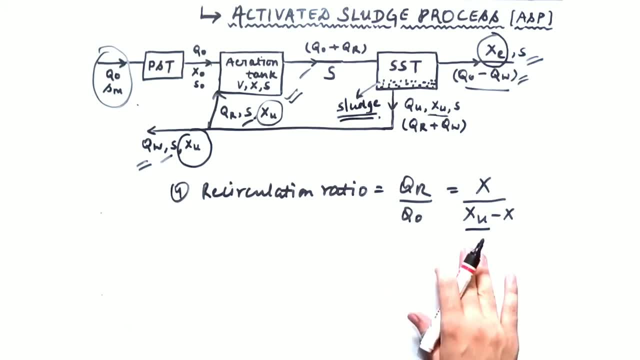 discharge and wastage discharge. So this is a very important formula. Sometimes you can ask for X, QR and Q0 and then ask for XU. So next formula is: Food by mass ratio, F by M. We have talked about this in detail. So what is food? Food. 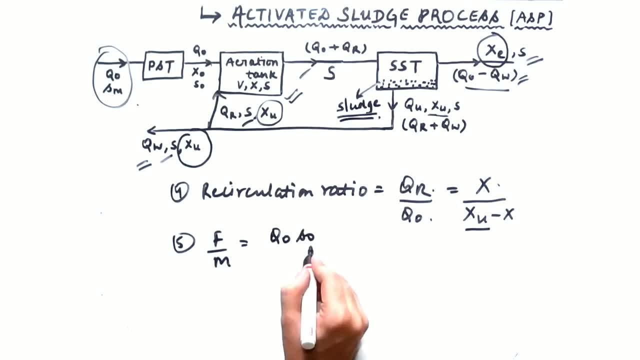 is Q0 into S0.. Q0 is coming and S0 is also coming, So this much organic content is available Here. we are not talking about utilization, So Q0 into S0.. What is mass? V into X? We have biomass. We have already seen V into X, So this formula is also very simple. Next, 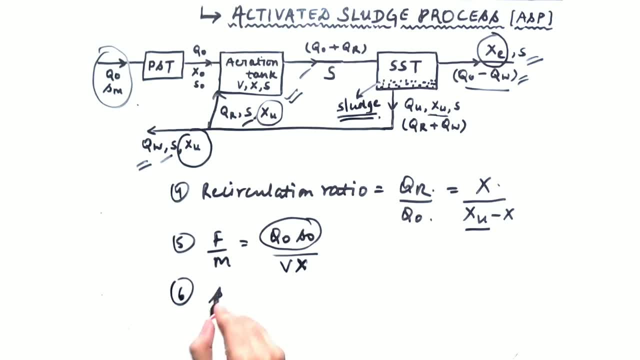 formula is sludge volume index. Now, this is a new term: Sludge volume index. Sludge volume index. What is this? See What is sludge volume index? basically, This is a parameter which tells the physical state of sludge solids. How dense are these sludge solids? 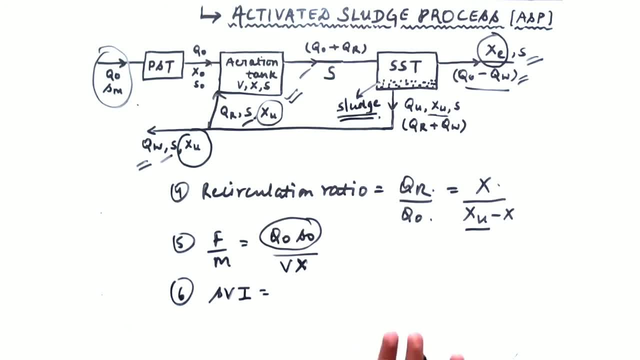 How much will they settle? The more they settle, the better it is for us, because our recirculated discharge concentration will be much better. So what do we do to get this out? We take a sample from the secondary sedimentation tank. We had a secondary sedimentation. 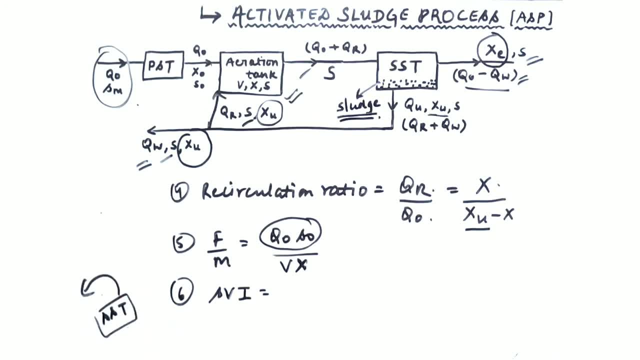 tank. We have SST. We took a sample from the secondary sedimentation tank. We took a sample from the secondary sedimentation tank. We extracted some samples from it. We take one litre of sewage sample from the secondary sedimentation tank. Now what we do is we let 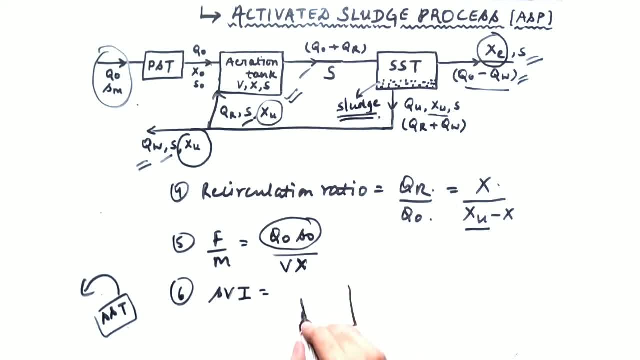 this sludge solid settle. We put this in a flask, We put this in and now we let it settle. We generally take a time of 30 minutes. This can be called a standard or thumb rule. We take a time of 30 minutes and we let it settle. So when it settles, we measure this sludge. 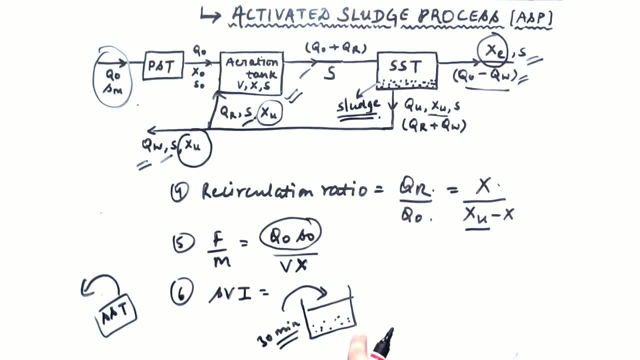 solids. We measure how much sludge solids volume we got in millilitres per litre We will get sludge volume, The sludge that we took below. we extracted it and we measured its volume. We have a lot of instruments to measure volume. So what we did is we measured. 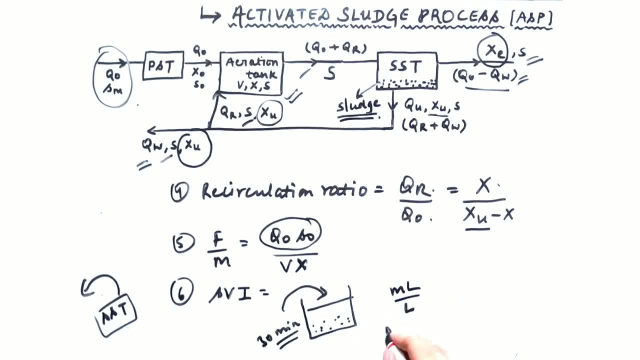 its volume in millilitres per litre, Divided by MLSS concentration. we measured. What is MLSS concentration? How much biomass do we have? So what we did is we measured the biomass concentration. What is biomass concentration? It is in milligrams per litre, So we divided. 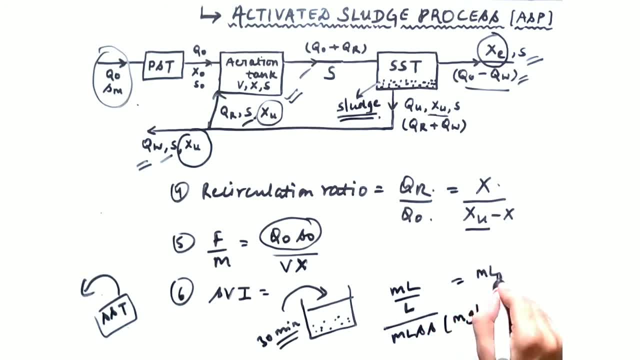 this. So what will we get? We will get SVI in millilitres per milligram, But its standard units are millilitres per gram. So you can convert milligram into gram by multiplying by 10 to the power minus 3.. So millilitres per gram will give you sludge volume index. 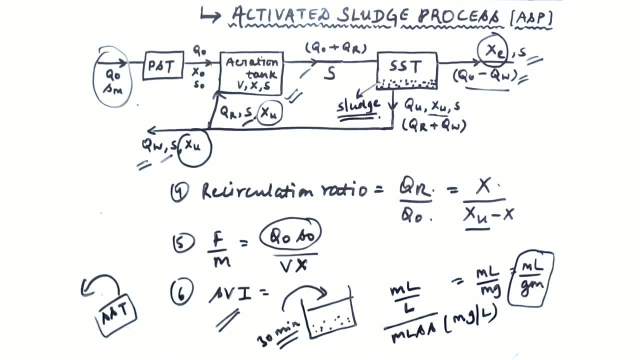 What was sludge volume index? You took some sludge from the secondary sedimentation tank to settle it. So you measured the volume of the sludge. that you got below because you took per litre So you have to take the volume directly, So millilitres per litre of the sludge. 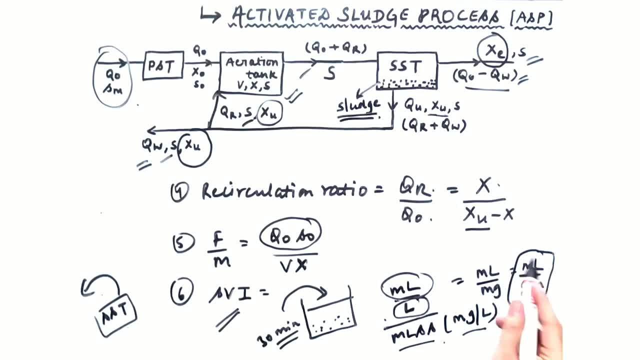 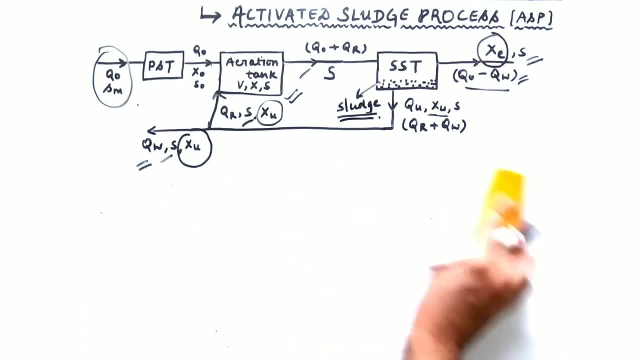 volume divided by MLSS concentration, which is in milligrams per litre, You will get the sludge volume index. You will get sludge volume index. I hope this is clear to you. The next formula is sludge density index, SDI. I hope this is the seventh formula. So you have sludge. 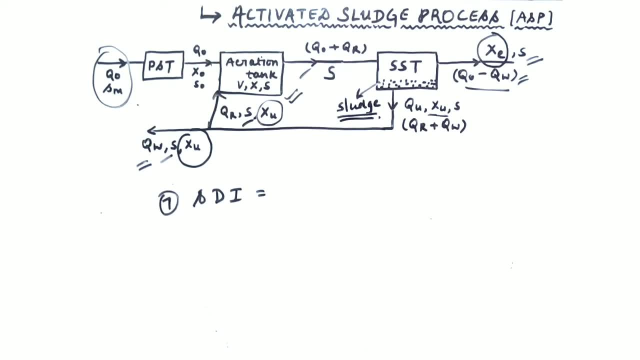 density index. So how will you get sludge density index? Simply, you have to do 1 upon SVI. You know what is the unit of sludge volume index, Millilitres per gram? I told you this is the standard unit. You have to convert it and take SVI in it. But the unit of sludge 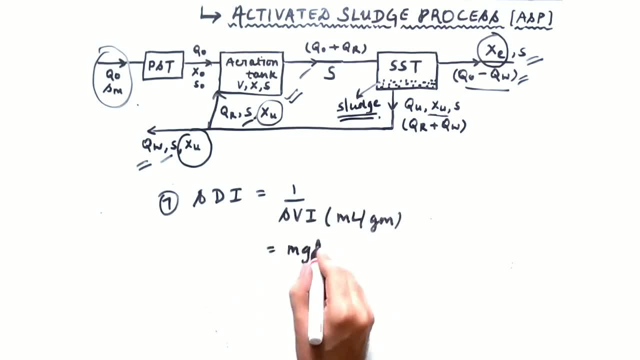 density index you have is in milligrams per litre. So you have to multiply it by 10 to the power 6 directly. Keep it in this unit. Keep SVI in millilitres per gram. You have to multiply it by 10 to the power 6.. So whatever answer you get will give you the sludge density. 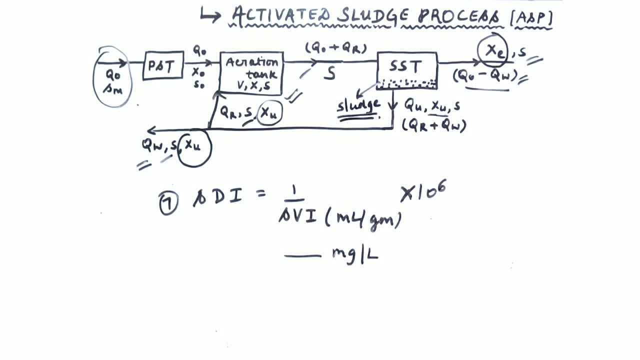 index value in milligrams per litre. I hope this point is clear to you. The next point is there is a small empirical formula And that is oxygen required in ASP. You have to give some oxygen in ASP If you know that the microorganisms which you feed in organic content. 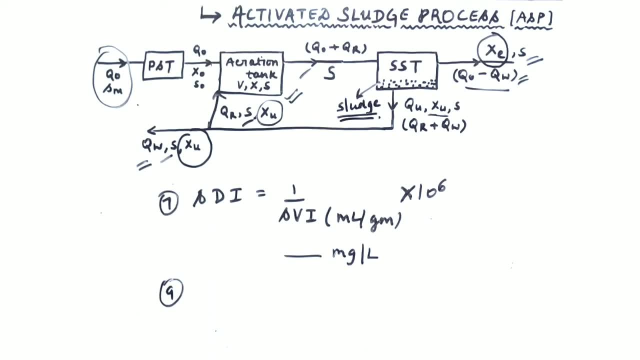 are aerobic microorganisms. They are not anaerobic, Because if they are anaerobic, then they will have end product alcohols and acids which we don't need. What we need is carbon dioxide. So what we do is we give some oxygen in it. It has an empirical formula: How much oxygen? 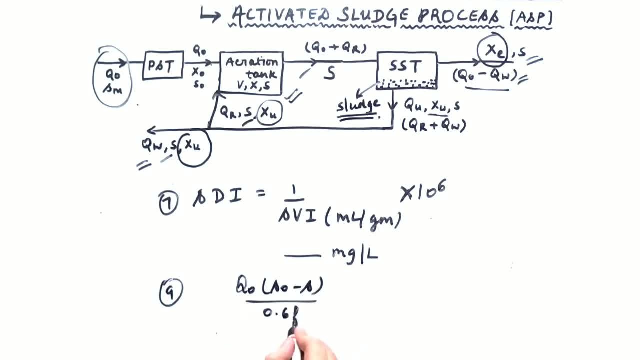 do we have to give in ASP Q0 into S0 minus S divided by 0.68 minus 1.42. QW into XU? What is this Oxygen required in ASP? This is an empirical formula. You can remember this particular. 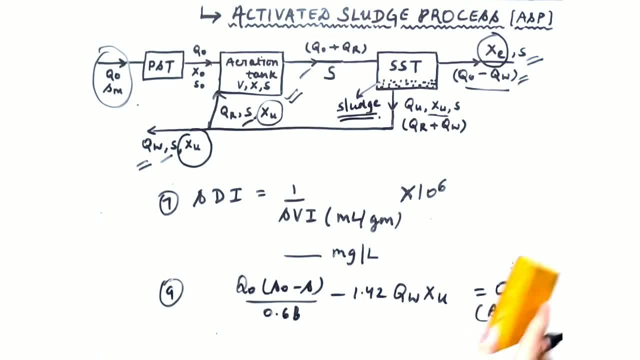 formula. So these are your formulas. Now you have two small equations which will come after the derivation. I will do the derivation, but the derivation is of not use at all. You should remember the end result of this derivation, And the end result is: K equals to QWXU divided by VX plus KER. What is KER? I will tell you. 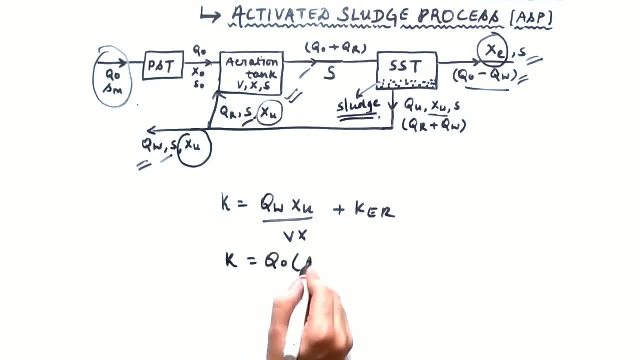 First you note the formula K equals to Q0, S0 minus S into Y divided by 0.68 minus 1.42 S into Y divided by VX. And one more very important formula in terms of theta C Is theta C S0 minus. 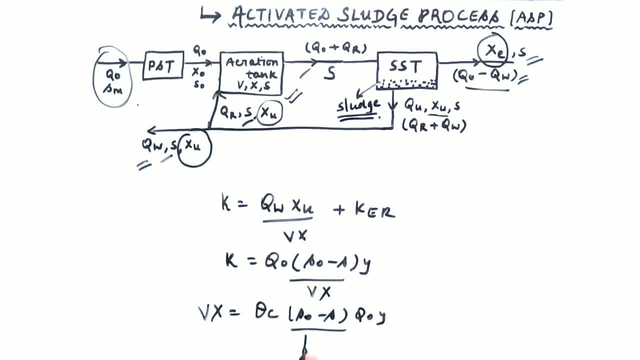 S, Q0 into Y divided by 1 plus KD. theta C. There is one formula of theta C. What is theta C? What is the age of your sludge, Or it is also called mean cell residence time, And this is also called sludge age. 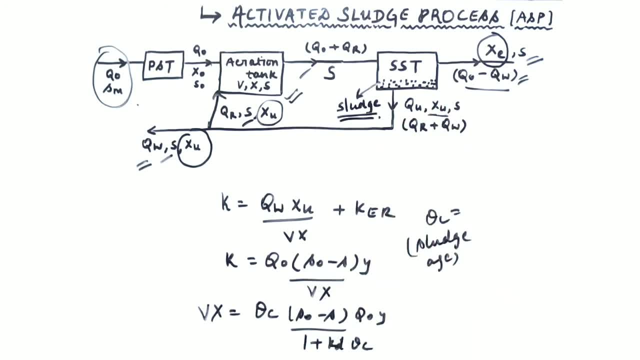 What is the age of sludge? What is the age of sludge? How long does sludge stay here? So what we do to find that out? VX is the concentration of biomass divided by Q0 minus QW into XE, plus QW into XU. 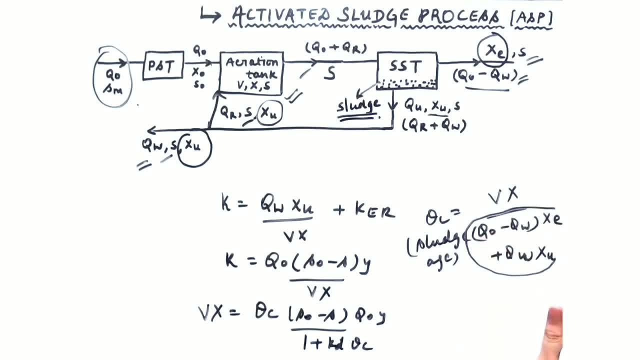 This is the MLSS concentration of the biomass which is going out. Q0 minus QW is going out here. You have multiplied it with XE. and this QW which is going out here, which is wasted, You have multiplied it with QW. 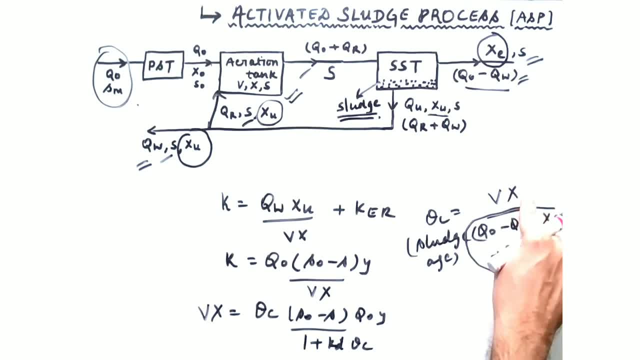 And this is in the denominator and in the numerator also, you will get MLSS concentration. So this will give you the age of sludge. This is also called mean cell residence time. This can also be asked in the question which has been asked. 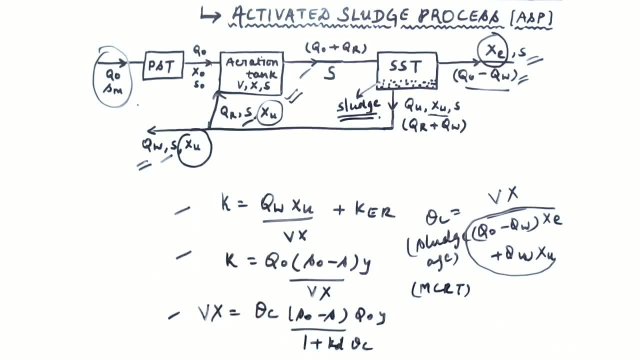 So you have three more equations which you can use. What is K? K is the deoxygenation constant. At what rate is the oxygen decreasing? This is called deoxygenation constant. You know the rest of the terms here. Only two terms are new for you. 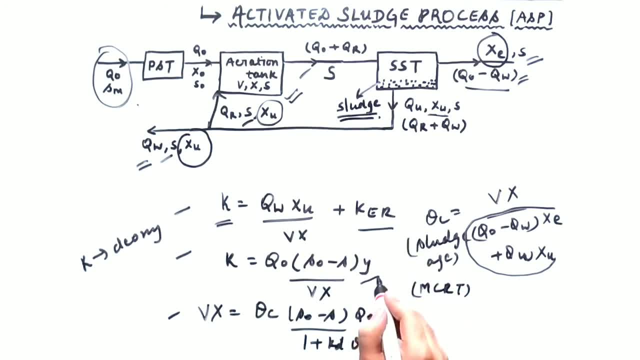 KER and Y. Let me tell you this: Y is basically the proportion of the biomass which is being produced in the MLSS concentration. Let me rub See What is Y Which is biodegradable. See, You have some organic matter. 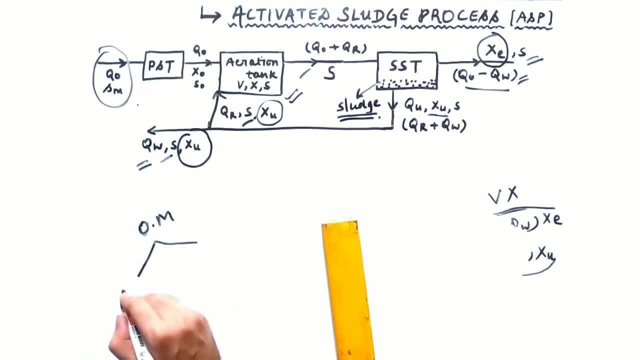 In this organic matter, some portion goes to the MLSS And some portion goes to your digested sludge. This means this will not give you any concentration of MLSS. So the proportion of organic matter which is being given to you by the MLSS- 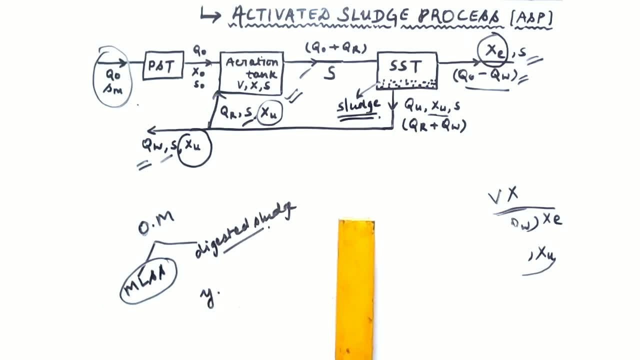 that is, the biomass, is called Y. I hope this point is clear to you. This is called Y And there was one more term there which we have read KER, So that KER is called as the endogenous decay constant. 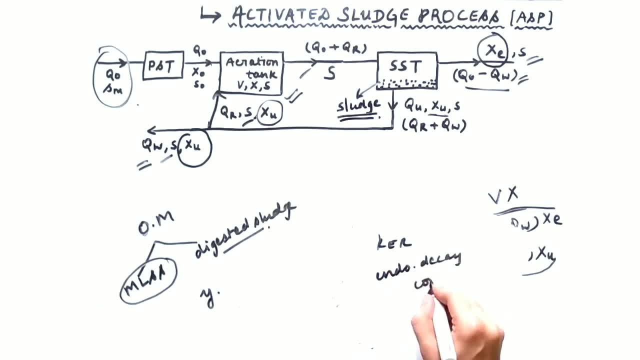 Endogenous decay constant, When you will read a graph from which you will get to know how your biomass is reduced- Sorry, How your food is reduced and how your biomass concentration changes. So this will be your graph. Here we have some phases. 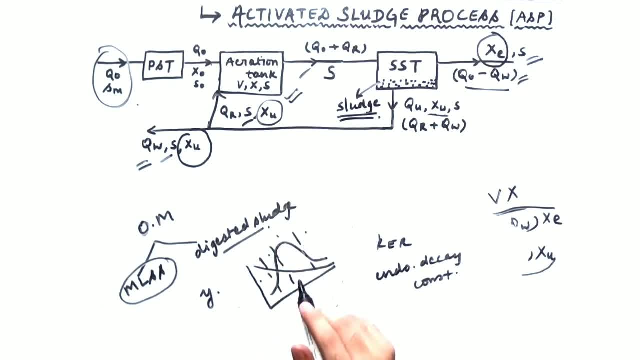 First phase, Second phase, Third phase And fourth phase. So the first phase we have is called lag phase. This is our first phase. This is called lag phase. In this the growth of micro-organisms is very slow. Micro-organisms are eating food very slowly. 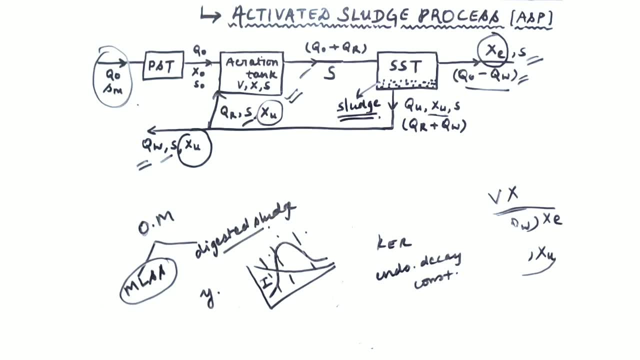 Because as soon as they get food they get accustomed to the type of organic matter And slowly their decomposition starts. This is called lag phase. Second is log phase. This is your second phase, Log phase, Log phase. Here you can see that the slope is very high. 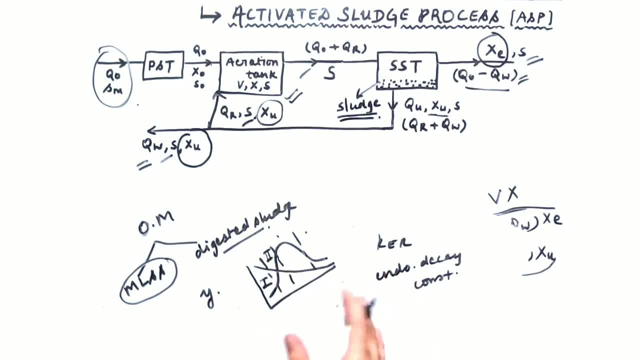 Here the micro-organisms are fully accustomed to the environment and organic matter, So the decomposition is very fast. This is our stationary phase. Third phase is called stationary phase. Here the rate starts to decrease gradually, Because the food will be finished gradually.